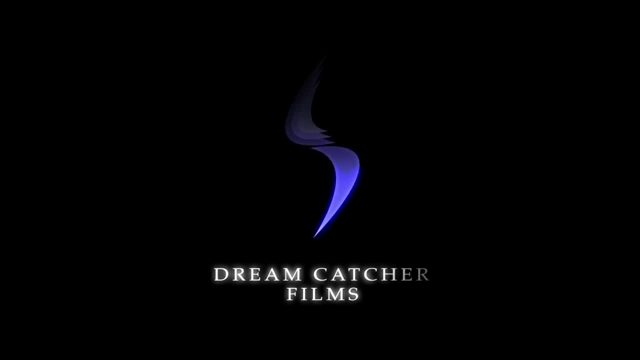 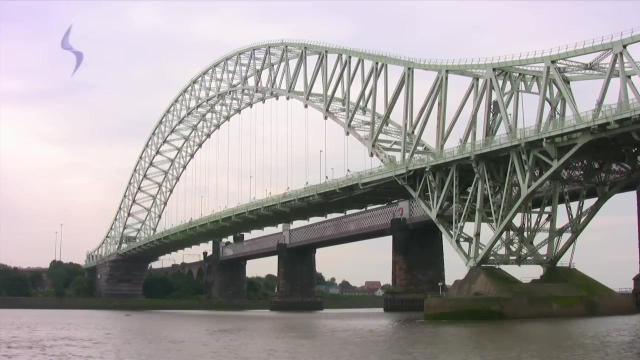 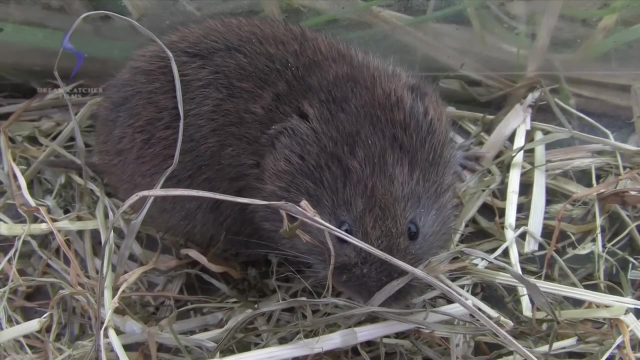 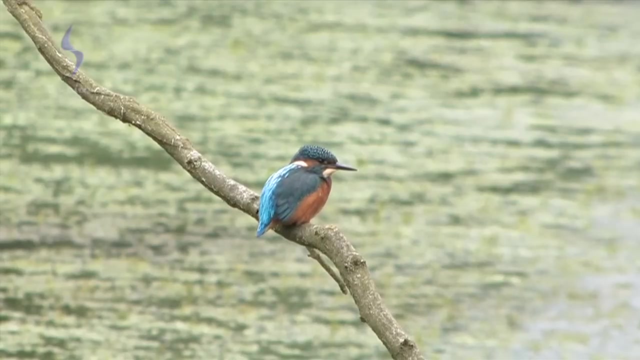 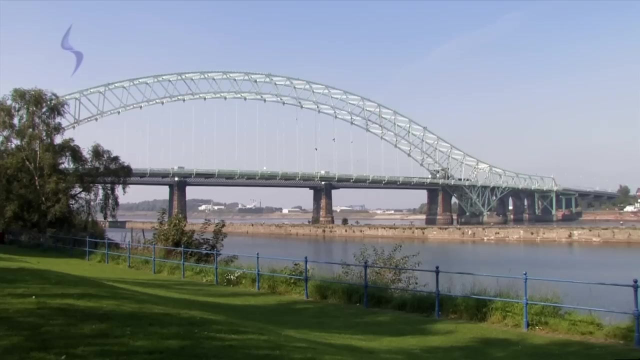 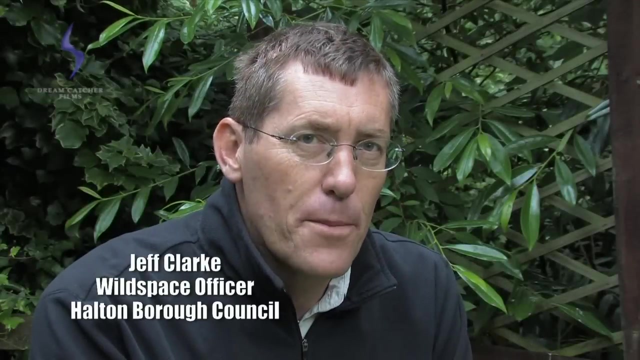 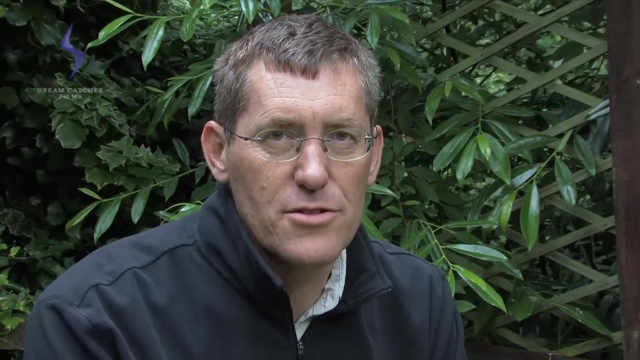 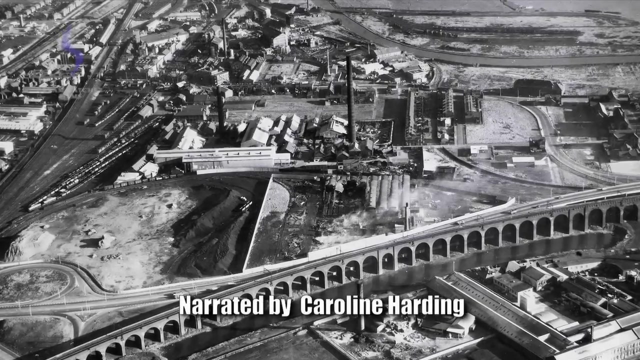 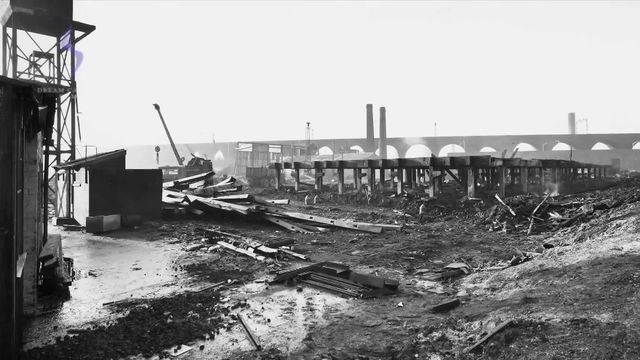 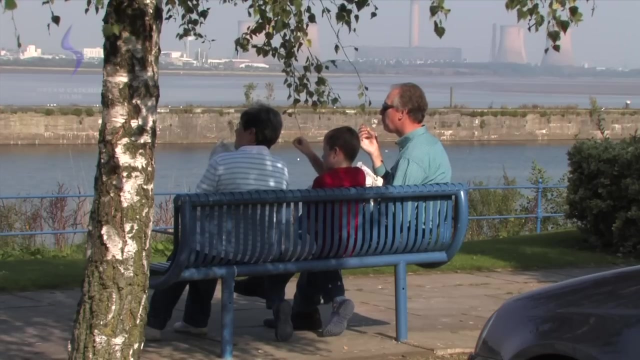 Thank you for watching. Thank you for watching can be both dramatic and devastating. Here in Halton we have a natural environment that has undergone a remarkable recovery from the dark days of the Industrial Revolution. That recovery and its impact on the species we feature. 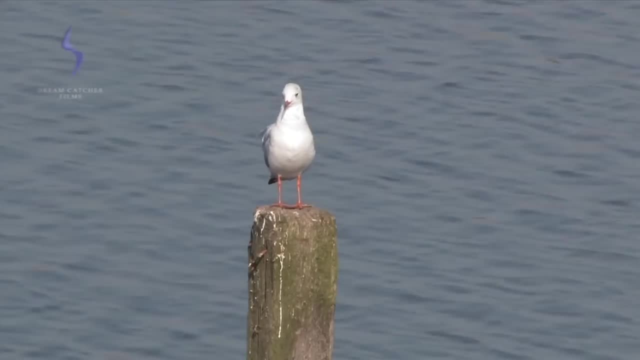 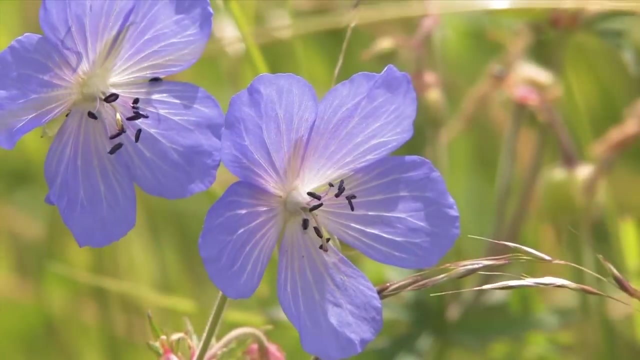 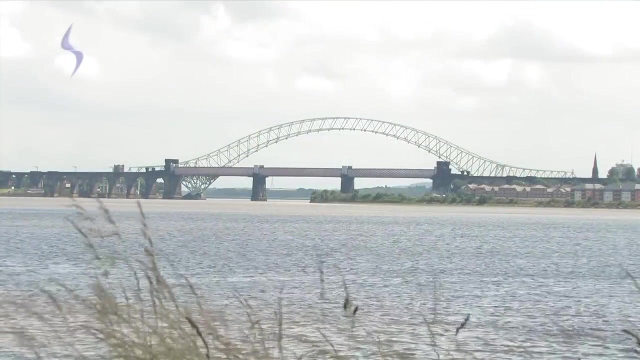 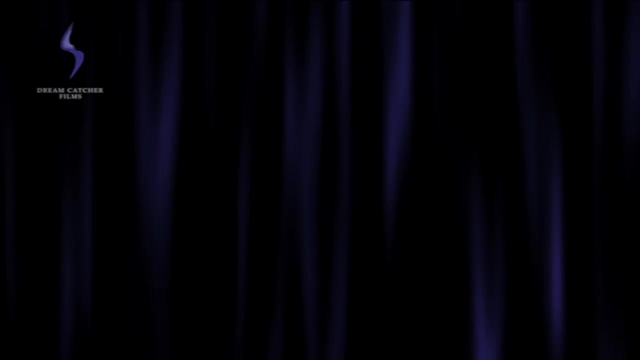 provide many clues that bring us to a better understanding of population dynamics and feeding relationships. Before we go any further, let's make sure you know some of the important things and important concepts in population dynamics and feeding relationships. Autotropes generate their own food from raw elements. 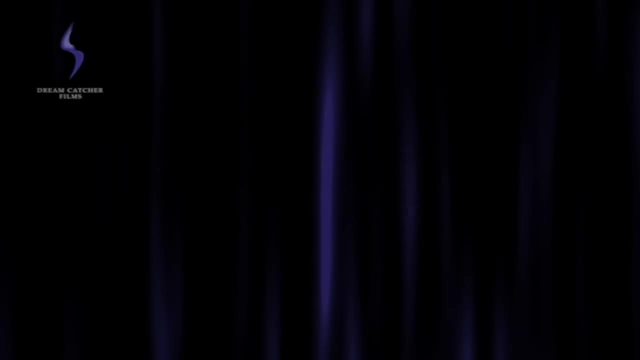 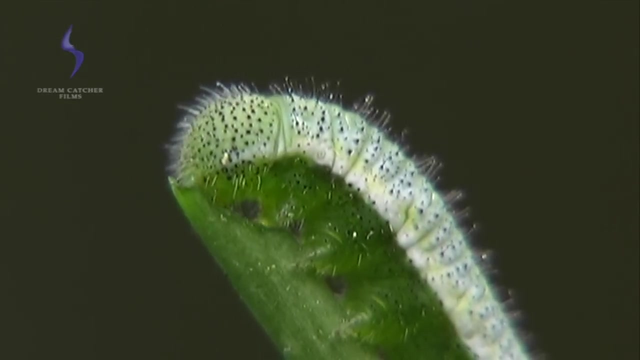 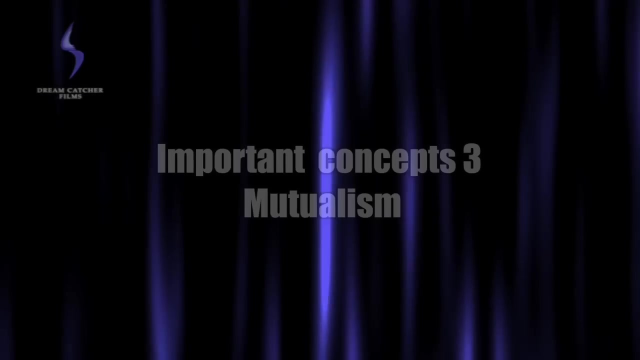 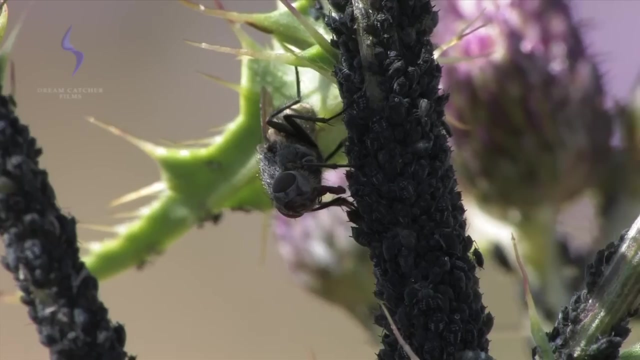 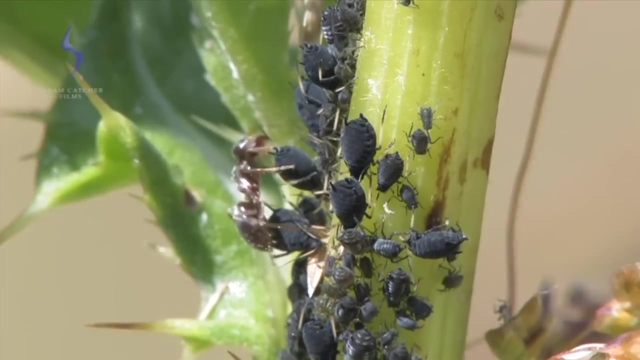 normally the power of the sun. Heterotropes ingest energy directly from other organisms, such as this caterpillar grazing That mammal is grazing on a stem. Mutualism: This is where two or more organisms benefit from a relationship. For example, ants milk aphids for their honeydew. 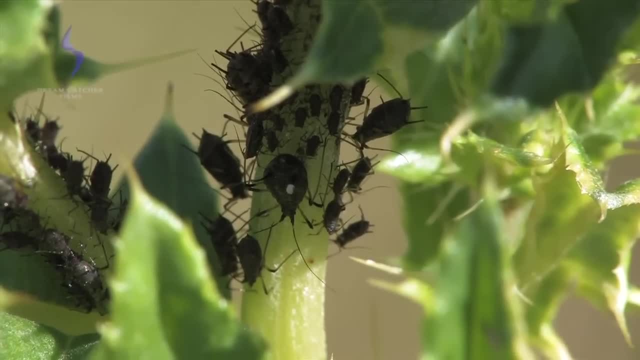 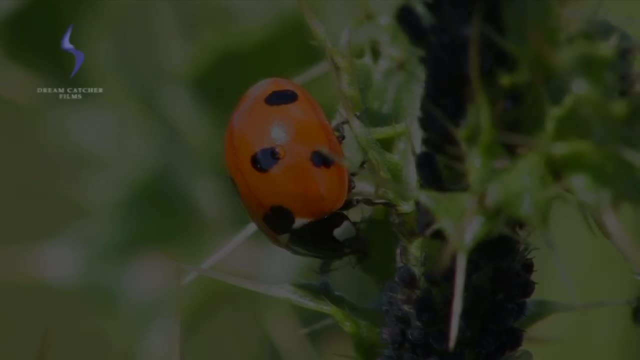 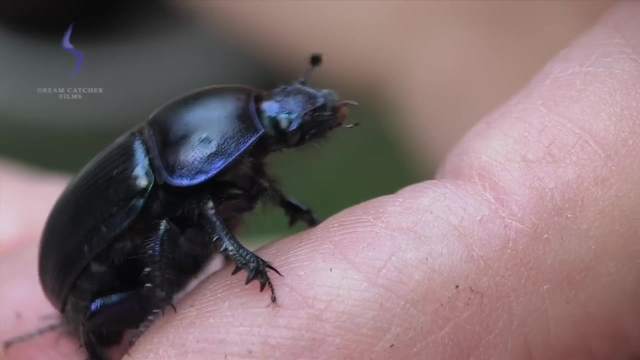 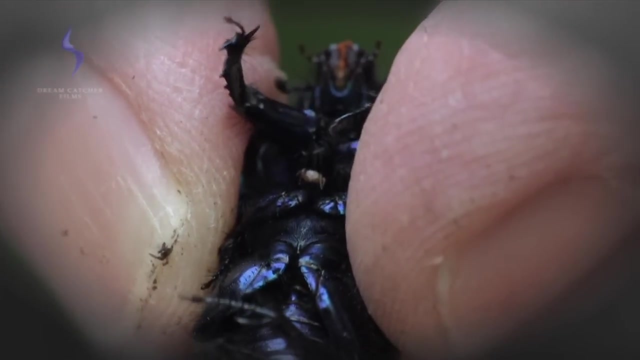 a sticky, sweet secretion. The aphids benefit because the ants defend them from potential predators like the ladybirds. Parasitism is a relationship in which one species benefits at the expense of the other. Here we can see a door beetle which is hosting a parasitic mite. 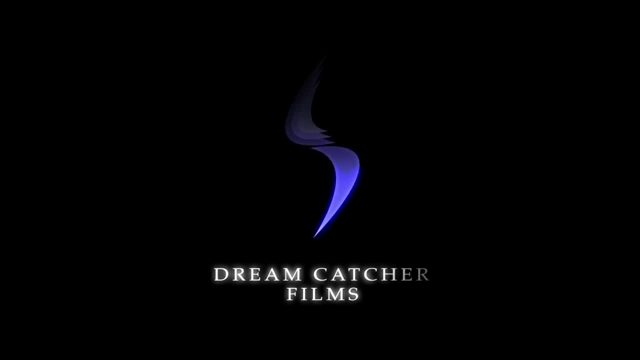 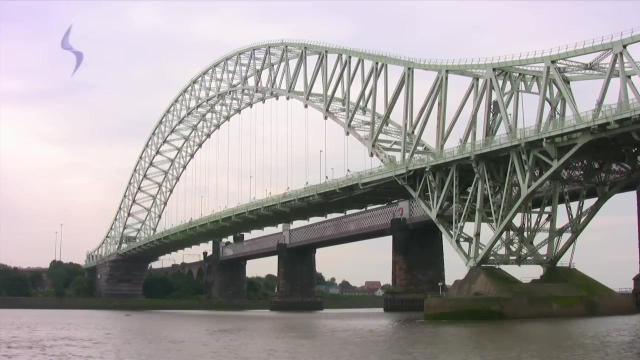 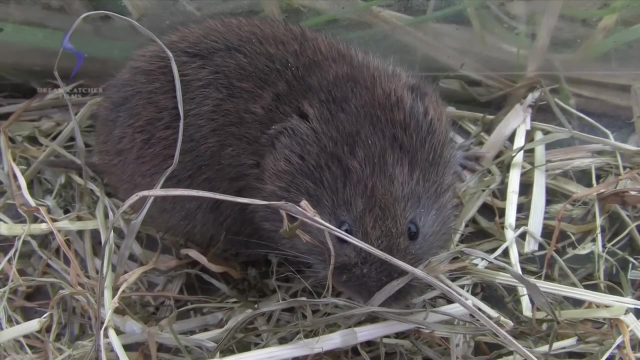 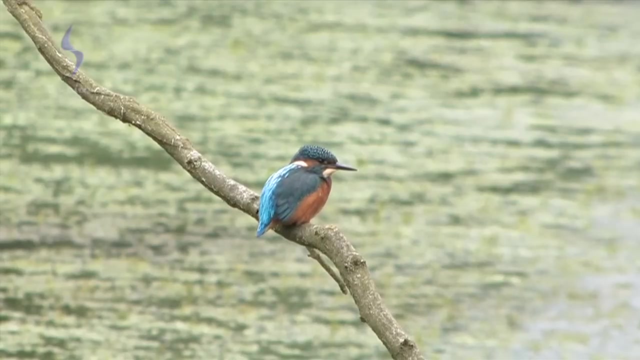 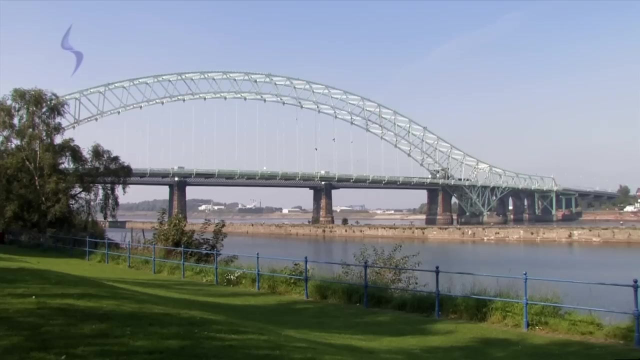 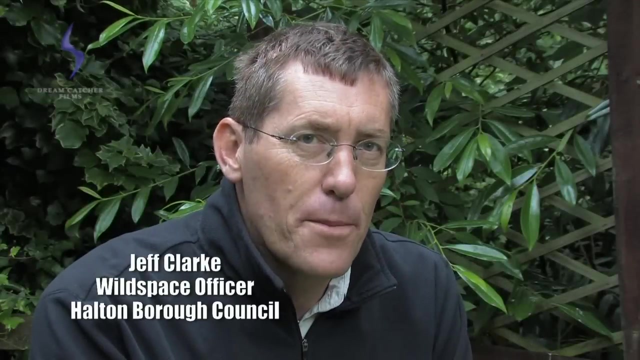 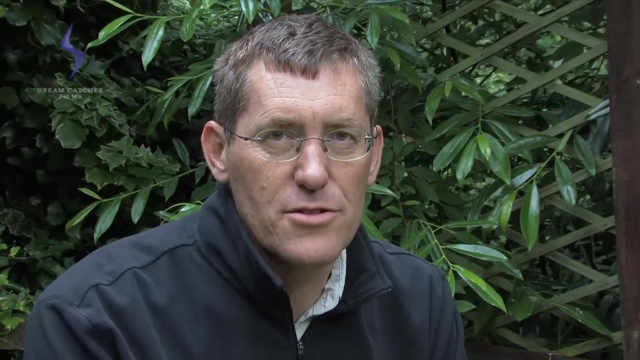 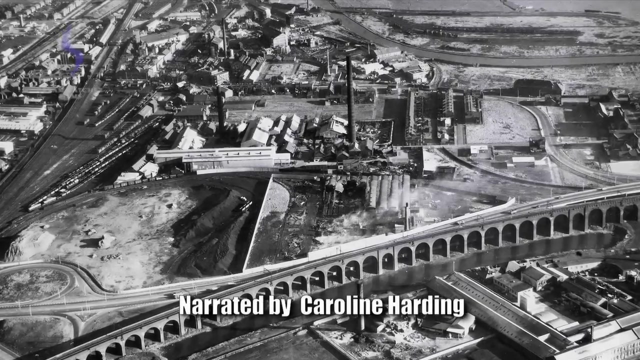 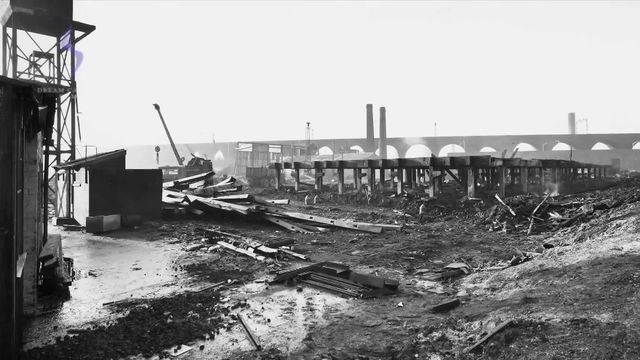 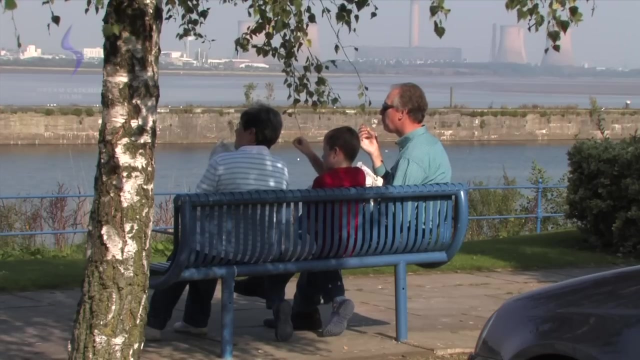 Thank you for watching. Thank you for watching can be both dramatic and devastating. Here in Halton we have a natural environment that has undergone a remarkable recovery from the dark days of the Industrial Revolution. That recovery and its impact on the species we feature. 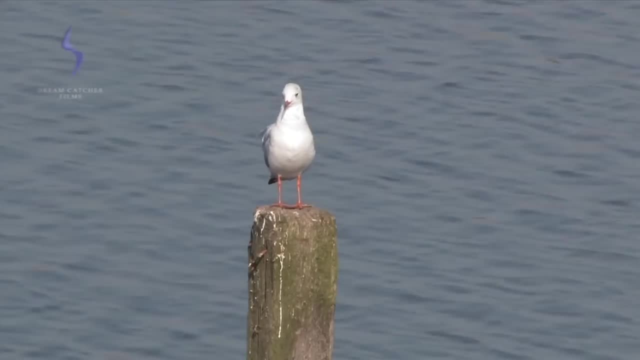 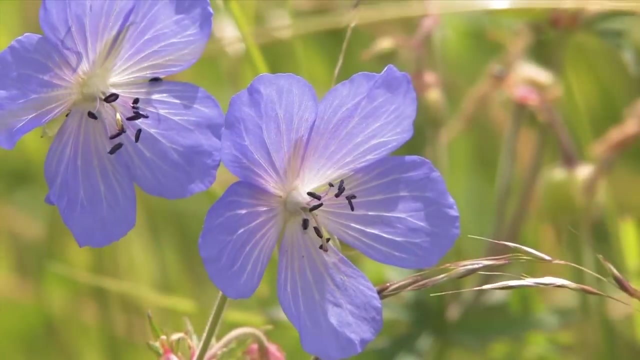 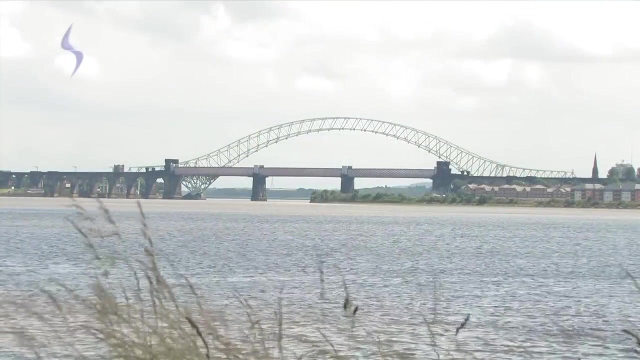 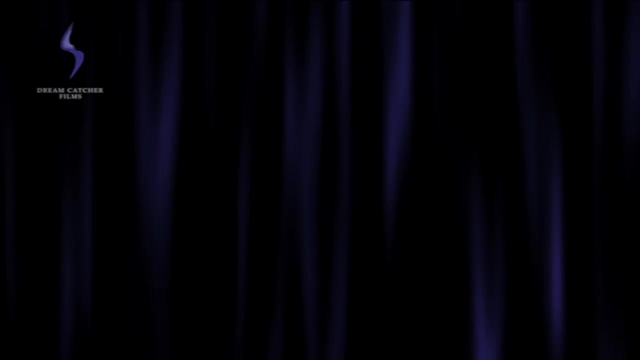 provide many clues that bring us to a better understanding of population dynamics and feeding relationships. Before we go any further, let's make sure you know some of the important things and important concepts in population dynamics and feeding relationships. Autotropes generate their own food from raw elements. 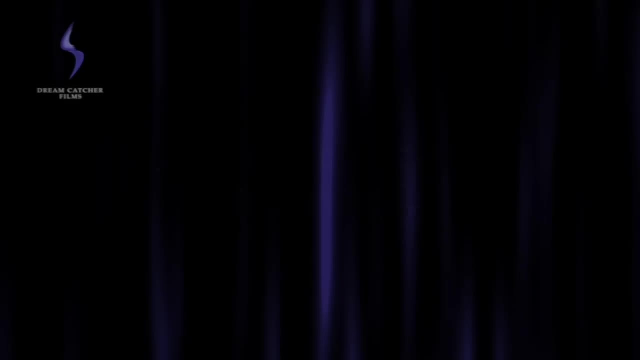 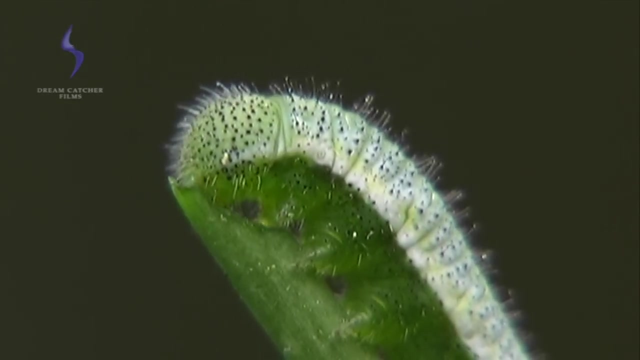 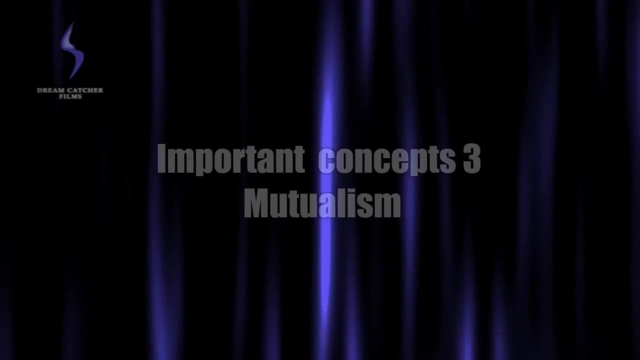 normally the power of the sun. Heterotropes ingest energy directly from other organisms such as this caterpillar grazing. The mother and the baby are the very first to lay their eggs in the egg nest. The eggs are the very first to be born and ready to be fed. 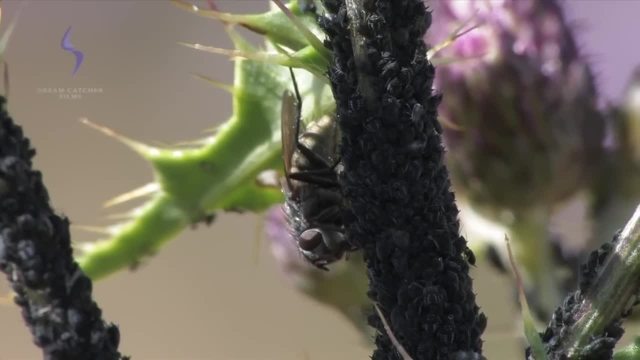 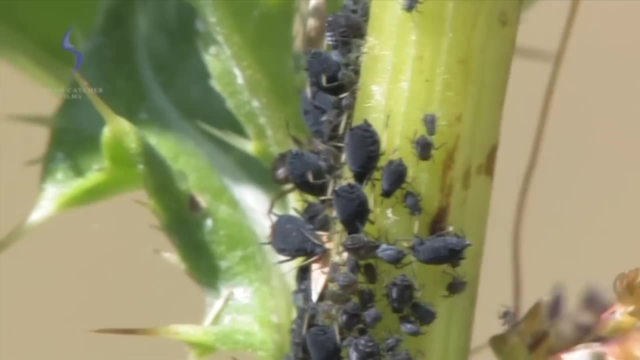 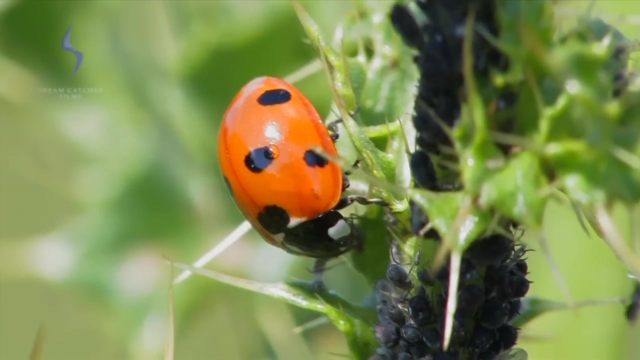 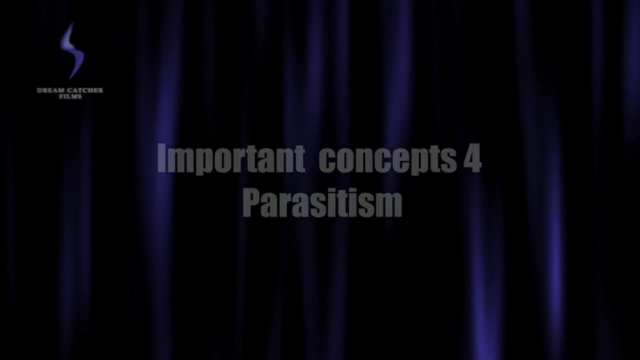 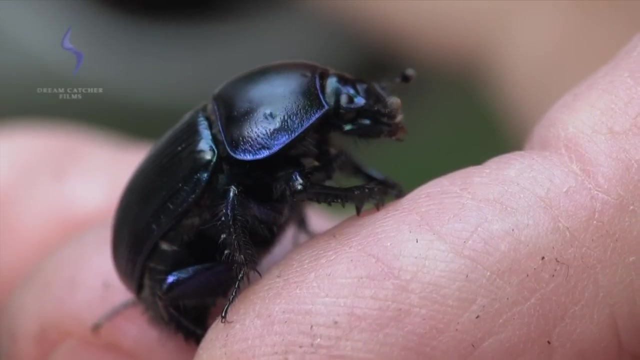 Mutualism: This is where two or more organisms benefit from a relationship. For example, ants milk aphids for their honeydew, a sticky sweet secretion. The aphids benefit because the ants defend them from potential predators like the ladybirds. Parasitism is a relationship in which one species benefits at the expense of the other. 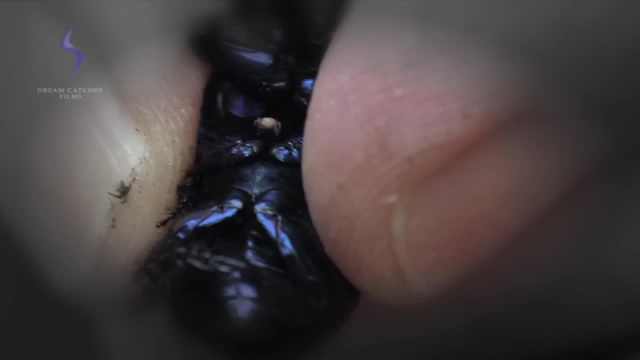 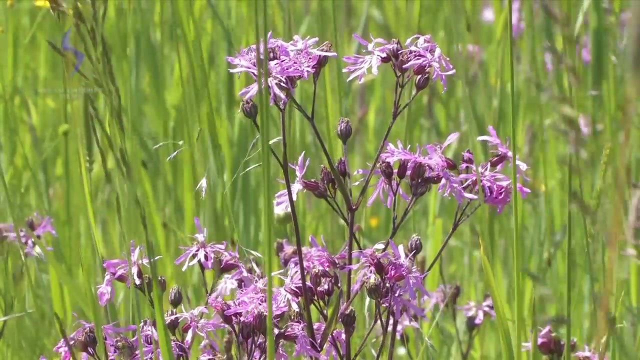 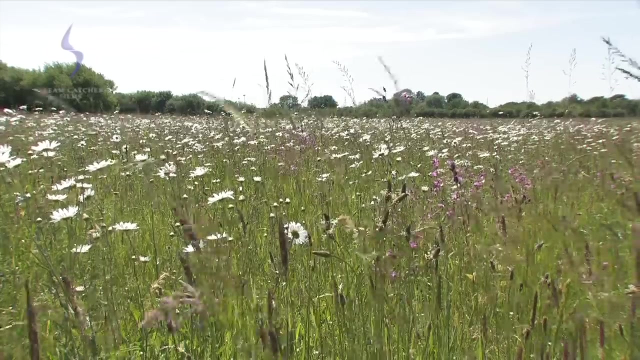 Here we can see a door beetle which is hosting a parasitic mite. Parasitic relationships can be devastating to the host species In honey bees. the recent collapse of many colonies has been caused by an accidentally introduced parasite, the varroa mite. 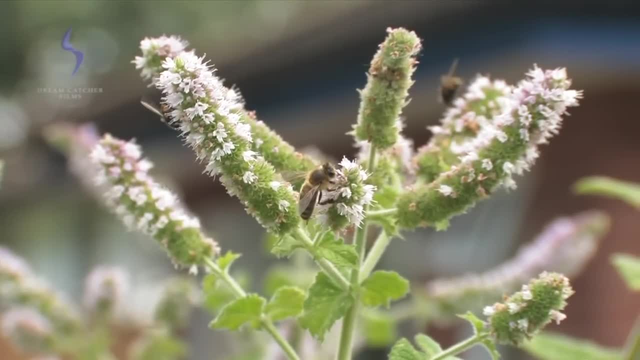 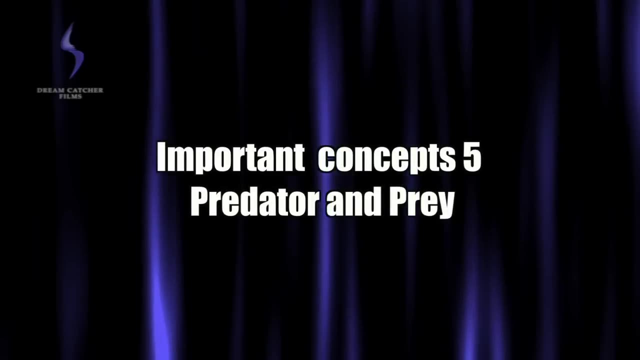 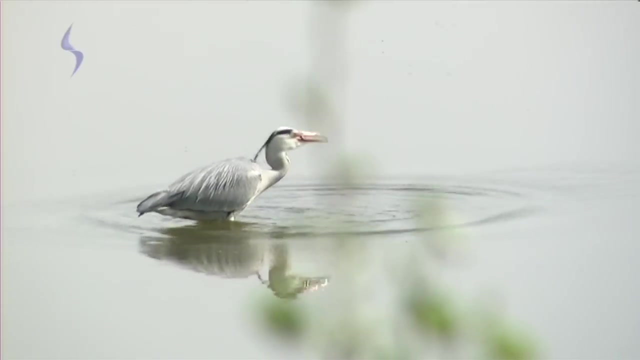 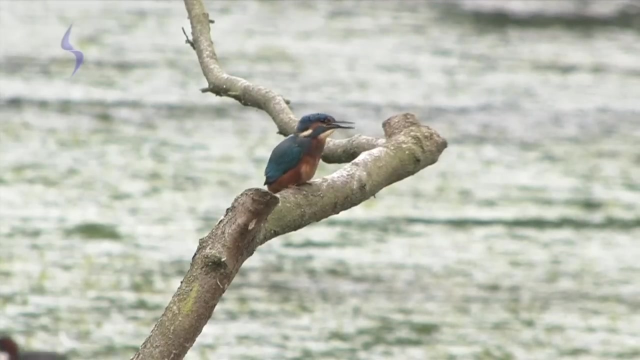 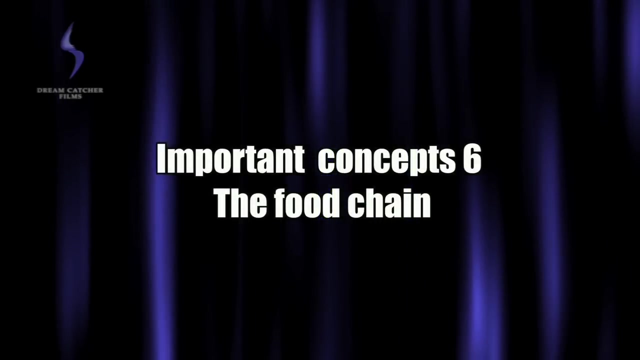 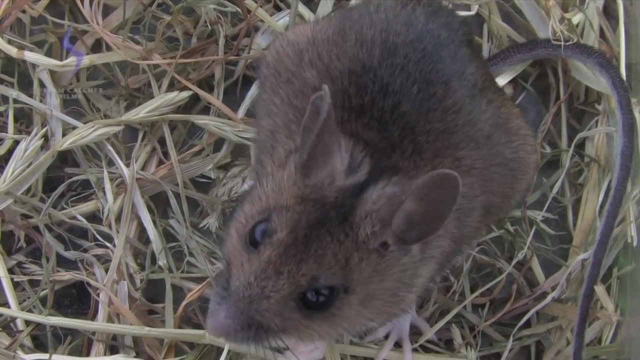 This has serious implications for our agricultural industry, as honey bees are crucial pollinators for many crops. Predation describes a biological interaction where a predator organism feeds on another living organism, or organisms known as prey. A food chain is a flow of energy from one organism to another in a community. 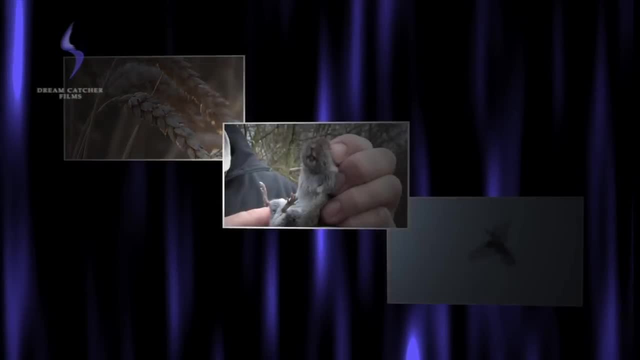 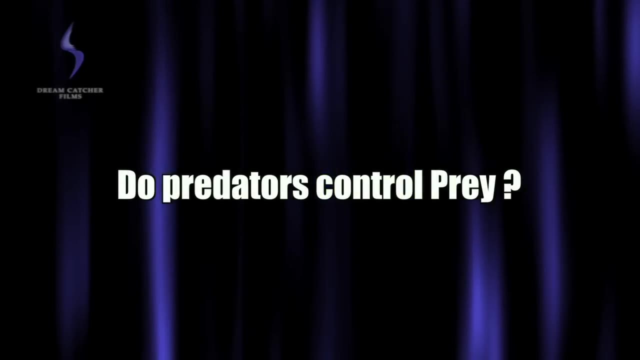 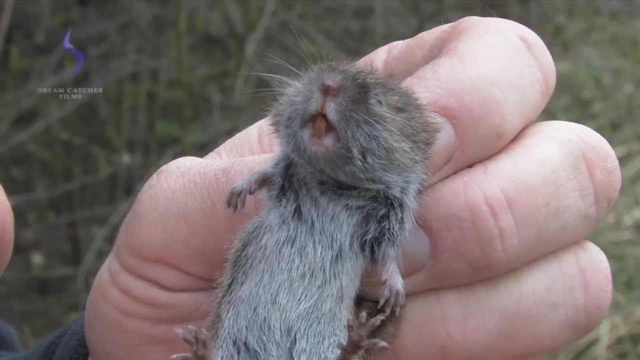 The producer is the grain, the primary consumer is the vole and the secondary consumer is the kestrel. This little fella is a short-tailed field vole. It's the main food of the common kestrel. It's going to help us answer the question: does the predator control the numbers of prey? 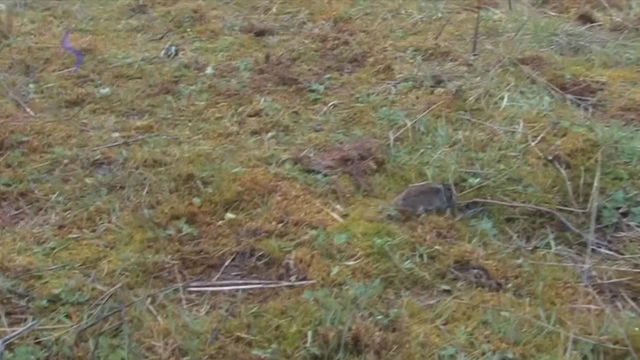 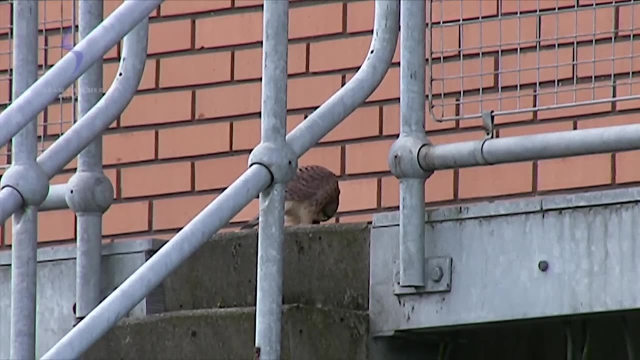 The obvious answer would seem to be yes. If a kestrel eats a vole, then it has reduced the total number of voles in a given area by one. In a year, a kestrel will eat the equivalent of 520 voles. 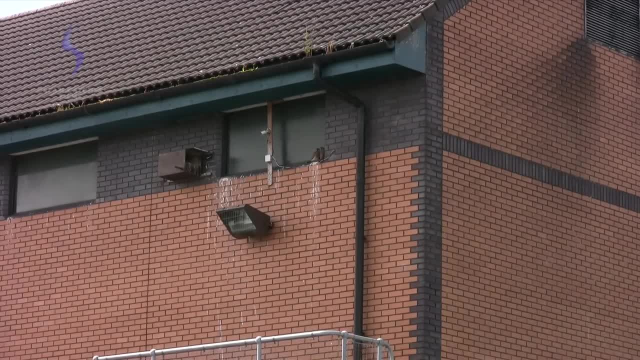 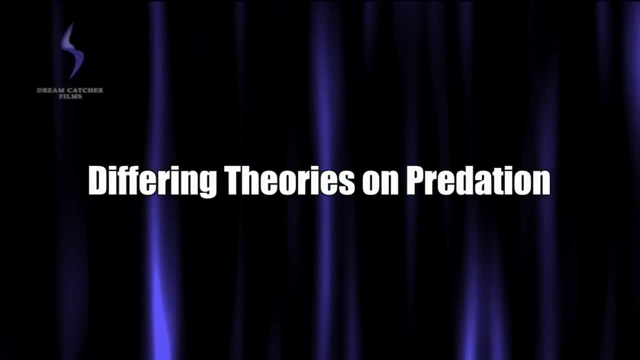 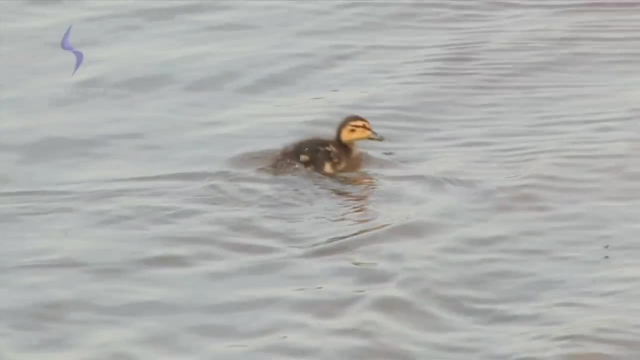 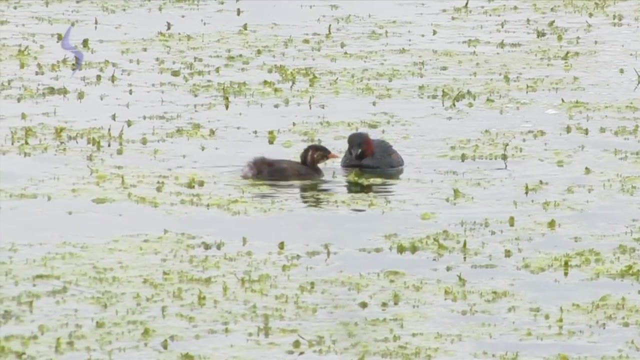 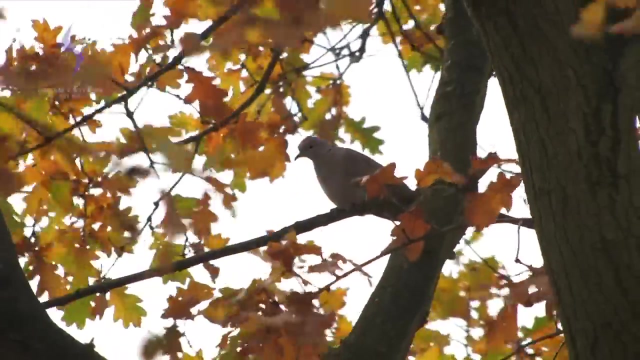 A pair and their four chicks will consume something like 1,400 voles from within their territory, The Hedgehog. Intuitively, we might guess that any predation will necessarily reduce the prey population size, But this is not necessarily true. Mortality caused by predation can be compensatory. Predation may compensate for mortality that would have occurred anyway. Due to competition, predation can also be compensatory. Due to competition, predation can also be compensatory weather or other factors, so that predation has no effect on population size. on the other hand, mortality due to predation can be additive taking. 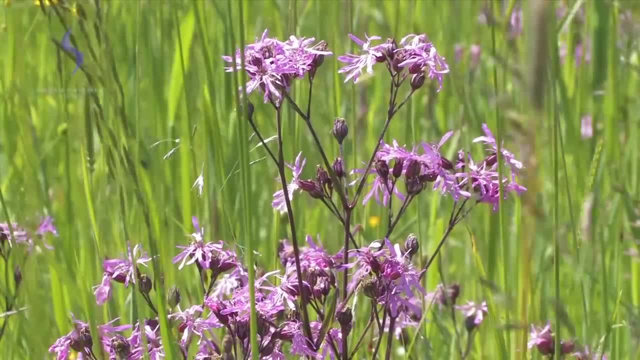 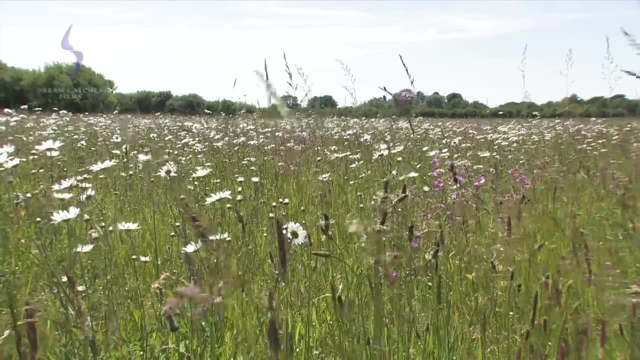 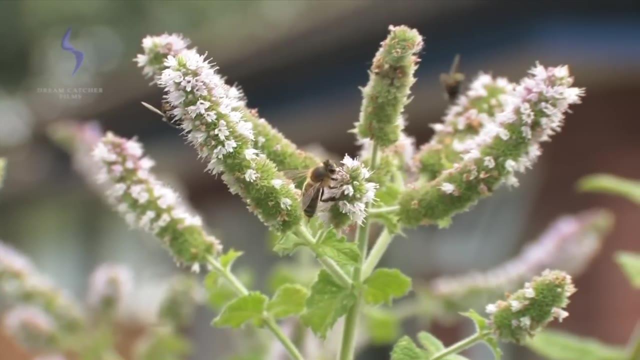 Parasitic relationships can be devastating to the host species. In honey bees, the recent collapse of many colonies has been caused by an accidentally introduced parasite, the varroa mite. This has serious implications for our agricultural industry, as honey bees are crucial pollinators. 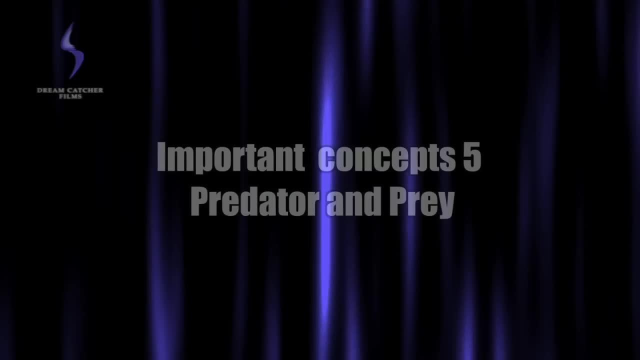 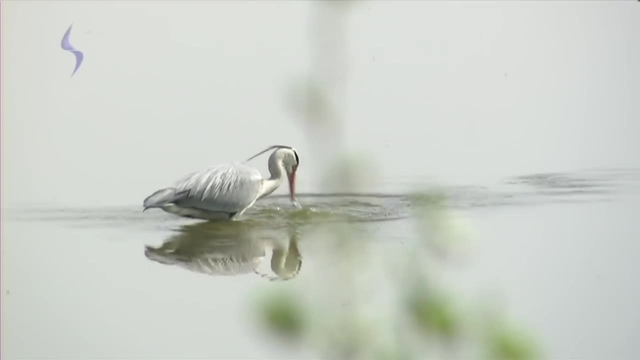 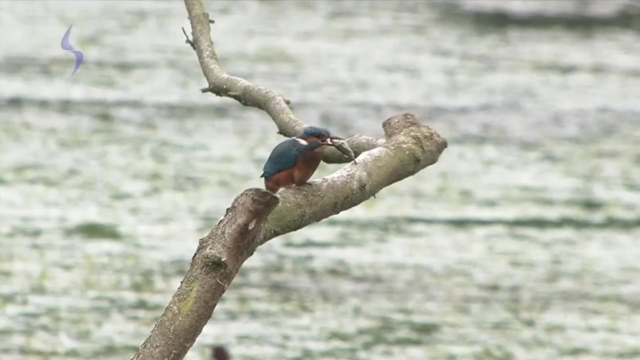 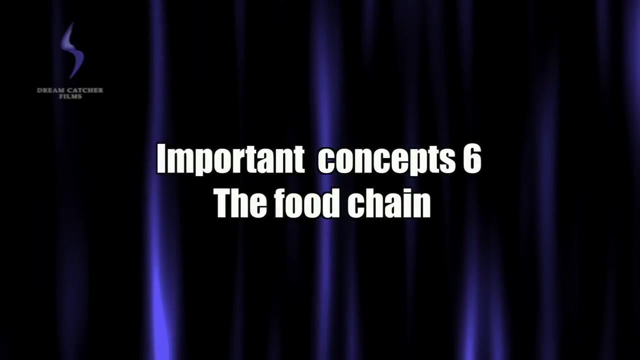 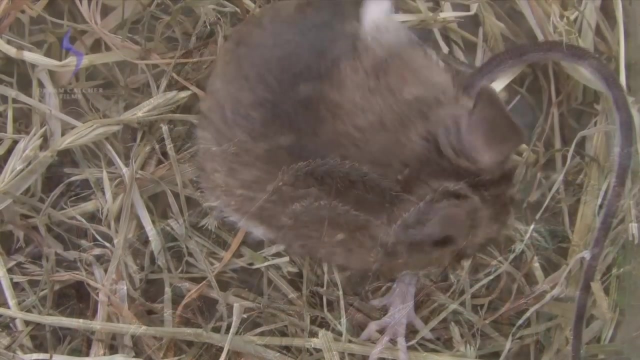 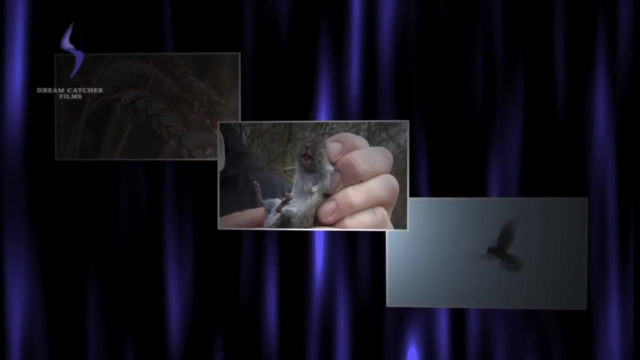 for many crops. Predation describes a biological interaction where a predator organism feeds on another living organism, or organisms known as prey. A food chain is a flow of energy from one organism to another. in a community, The producer is the grain, the primary consumer is the vole and the secondary consumer is 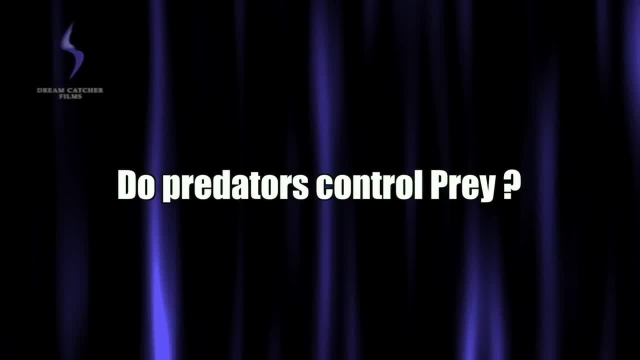 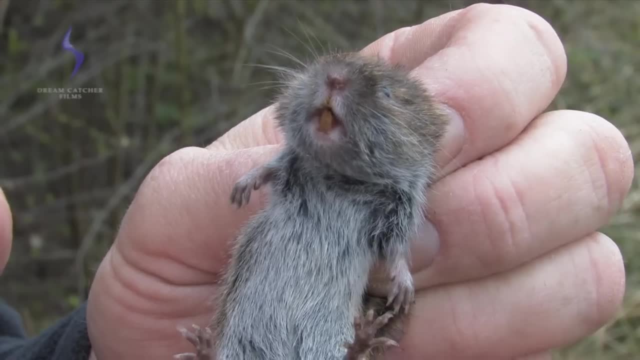 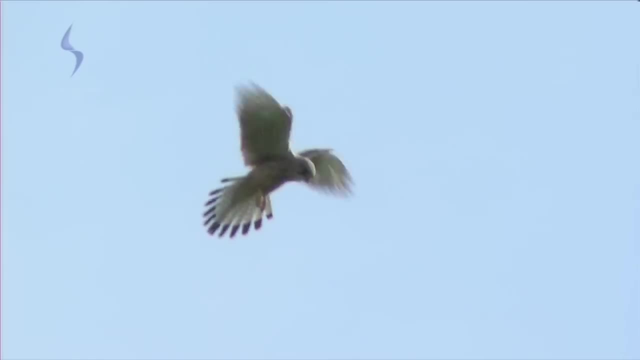 the kestrel. This little fella is a short-tailed field vole. It's the main food of the common kestrel. It's going to help us answer the question: does the predator control the numbers of prey? The obvious answer would seem to be yes. 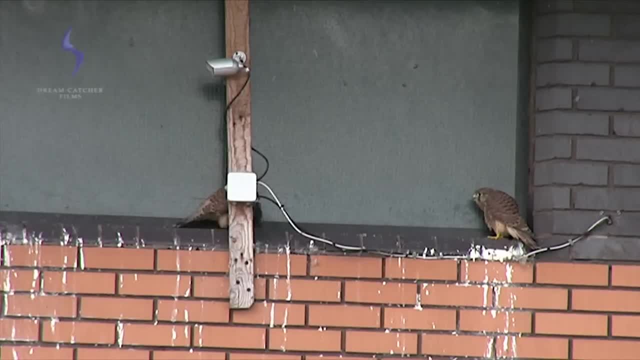 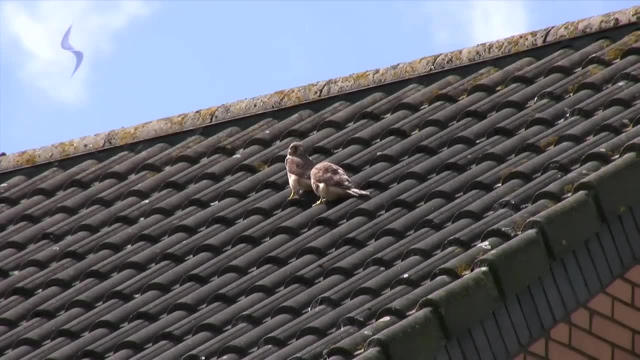 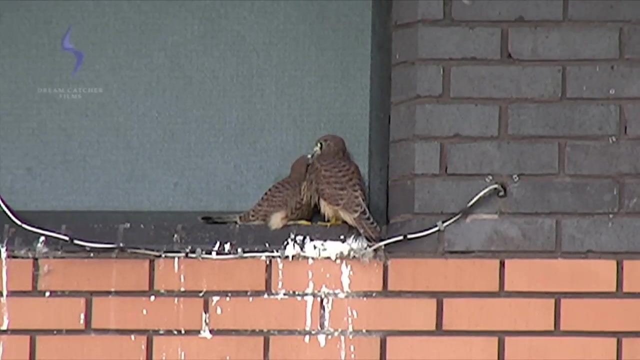 If a kestrel eats a vole, then it has reduced the total number of voles in a given area by one. In a year a kestrel will eat the equivalent of 520 voles A pair, and their four chicks will consume something like 1,400 voles from within their 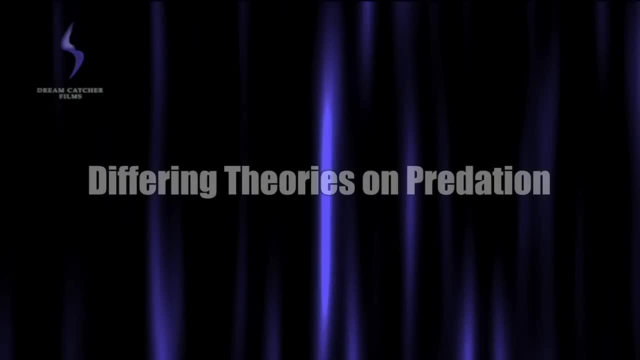 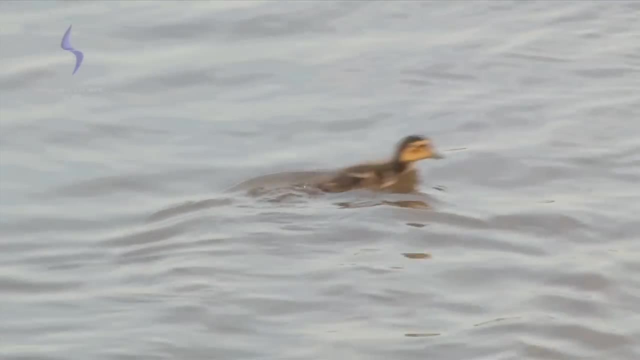 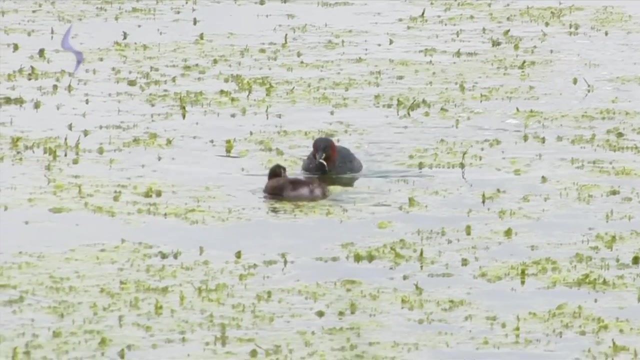 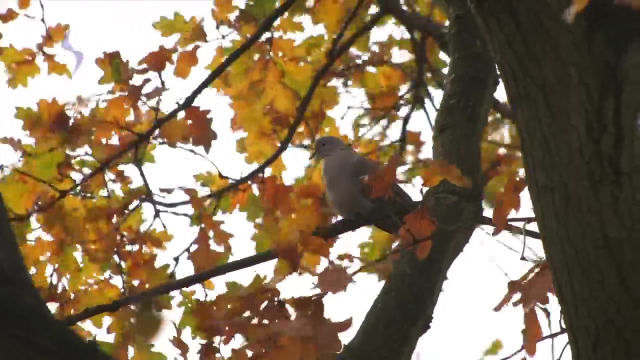 territory. It is to be expected that the predatory system will be able to control the number of voles every year. Intuitively, we might guess that any predation will necessarily reduce the prey population size, But this is not necessarily true, For example, if the predator has a full-fledged population and has a minimum food source. 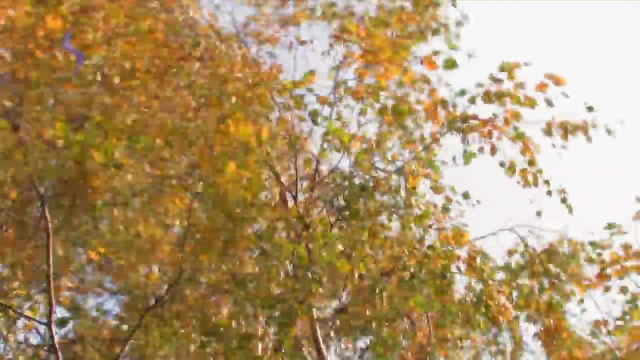 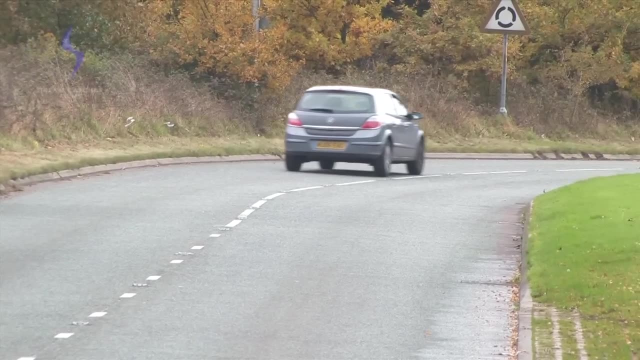 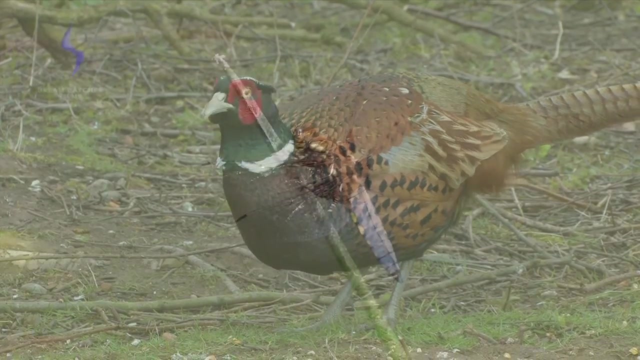 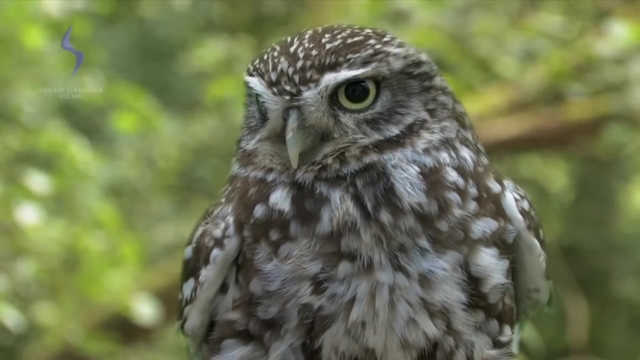 it will have to make a habit of getting the most feed for the whole population in order to take over weather or other factors, so that predation has no effect on population size. on the other hand, mortality due to predation can be additive, taking individuals that would not have died for other reasons. if this happens, the prey 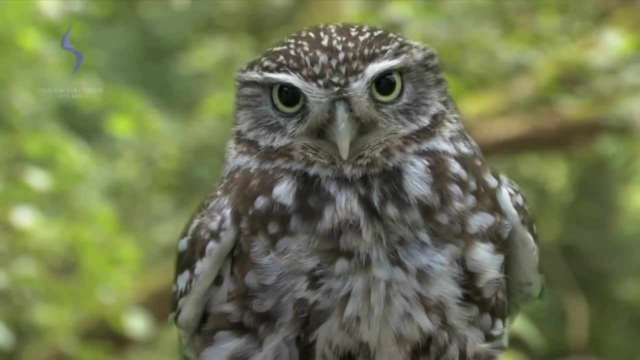 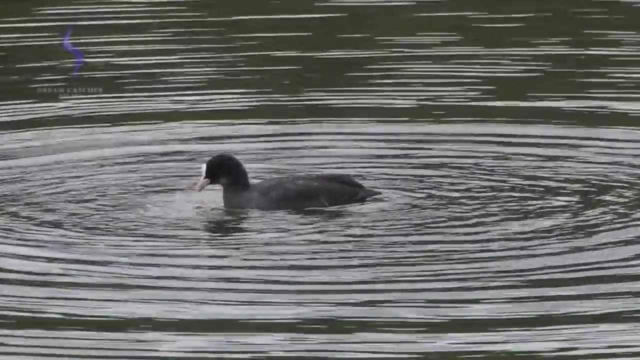 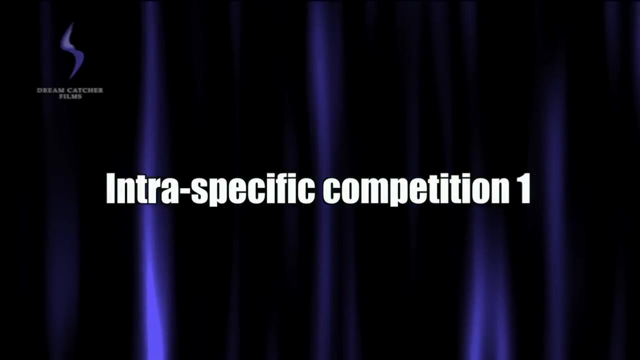 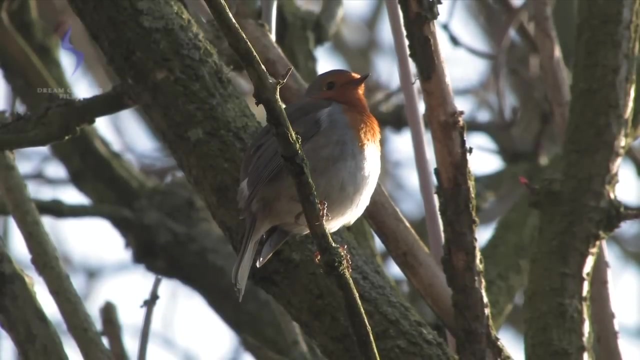 individuals that would not have died for other reasons. if this happens, the prey population growth rate will be affected, unless it can be compensated by a reduction in intraspecific competition. what is intraspecific competition? this occurs when two or more individuals of the same species strive for the same resource. this is easily observed, as it 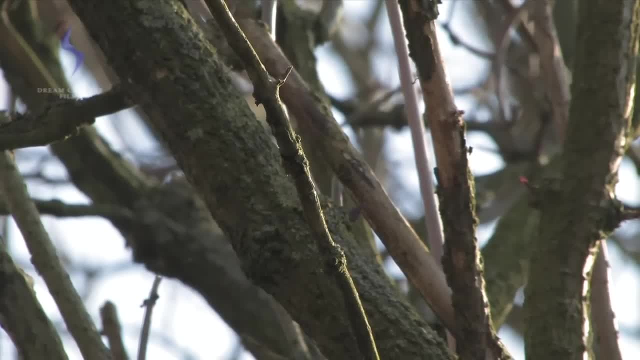 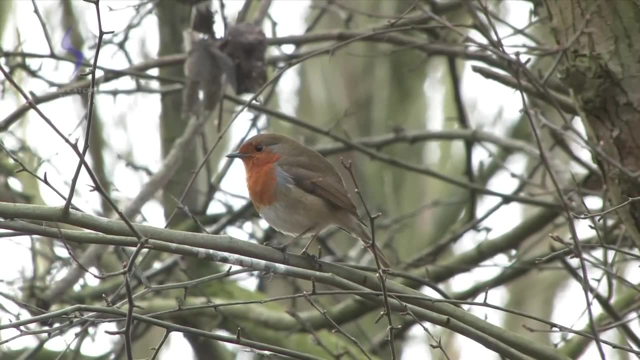 often leads to very visual or noisy contests. many species become territorial in defense of their species and in defense of their species and in defense of their valuable food resources. robins are an obvious example of this sort of behavior. birdsong is an audible expression of this contest for resources. similarly, 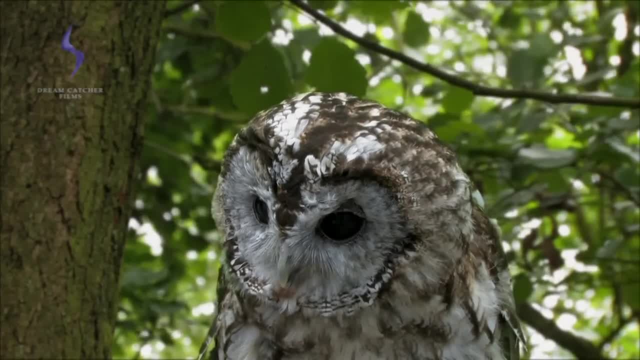 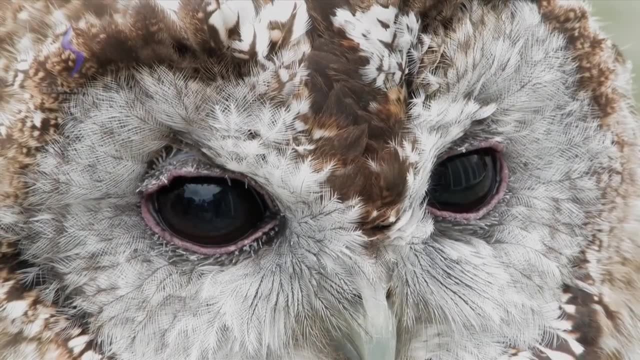 tawny owls are fiercely territorial. they pair for life and defend their breeding area against all other tawny owls in order to secure the food resources and nesting sites. at the population level, intraspecific competition is a very important factor in the survival of birds and in the survival of animals. the 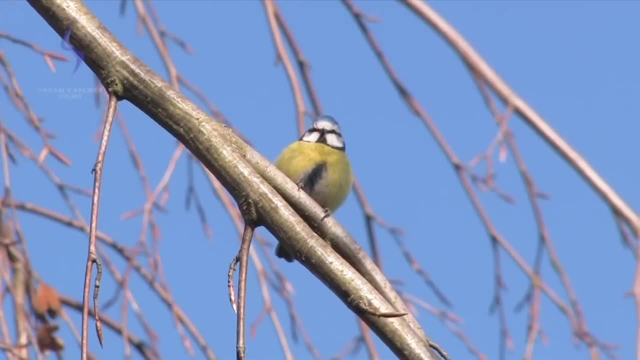 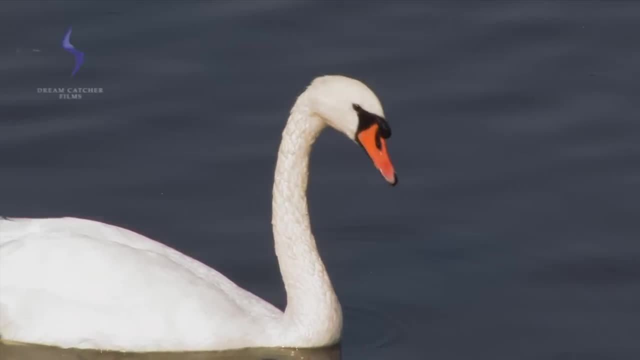 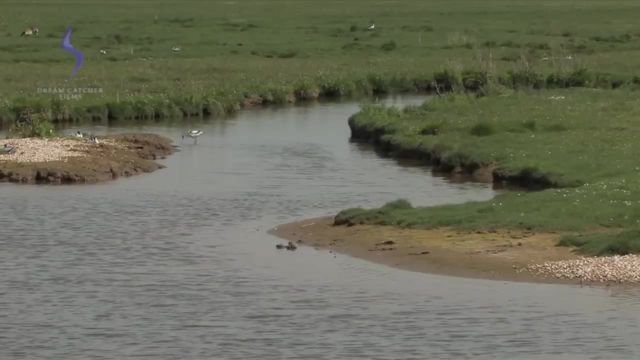 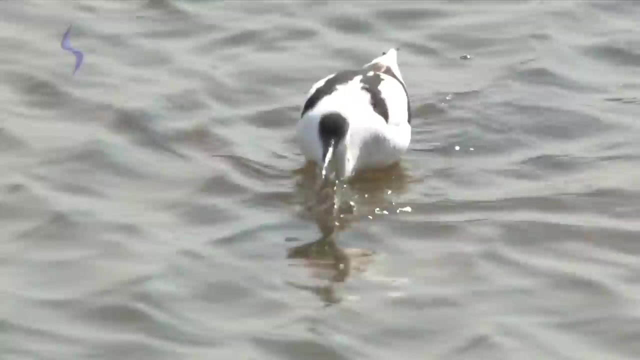 intraspecific competition for resources can bring about the overall decline in population of an organism when it exceeds the carrying capacity of its environment. carrying capacity is defined as the maximum number of individuals of a given species that a site can support during the most unfavorable time of year without. 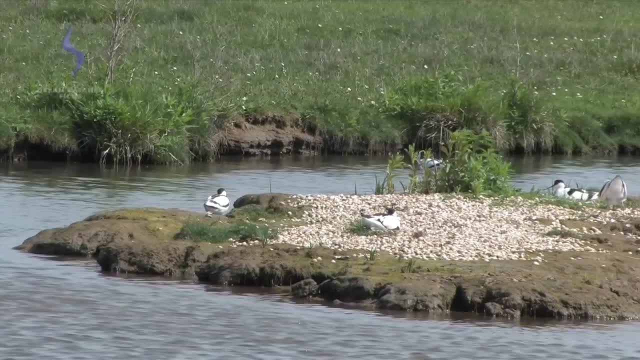 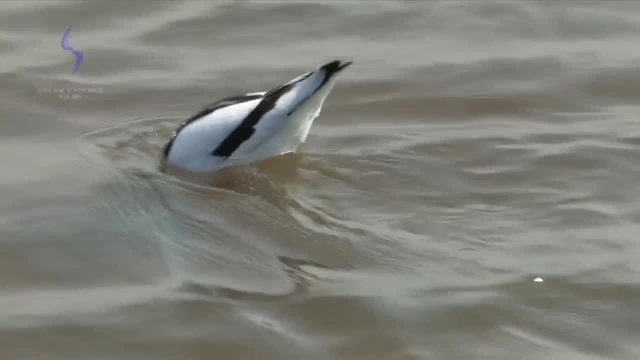 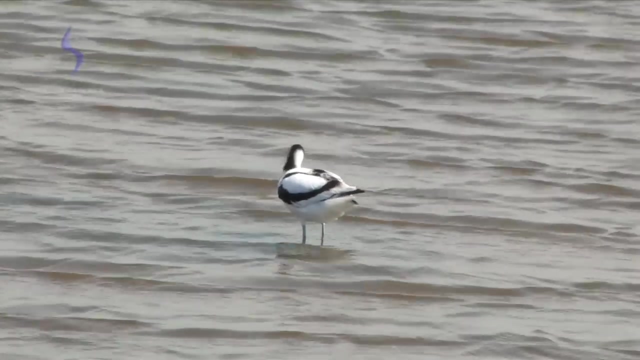 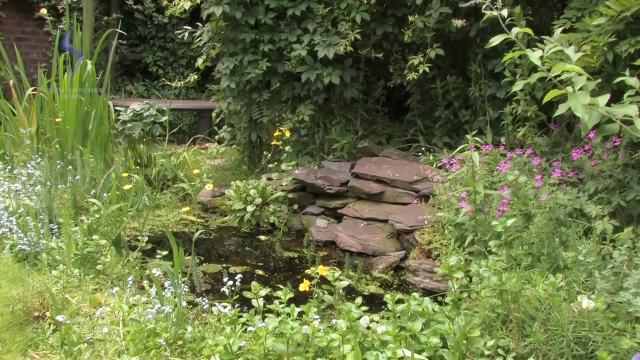 causing deterioration of the site. this is what would determine the maximum number of avocets that can be supported on breeding lagoons, feeding on small aquatic invertebrates without reducing their ability to find enough food to sustain them. lecking is one of the more extreme examples of visible intraspecific 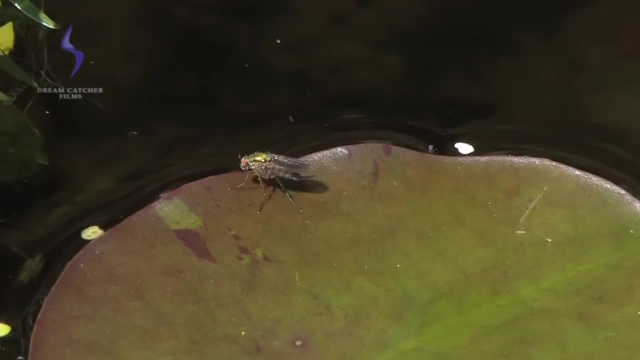 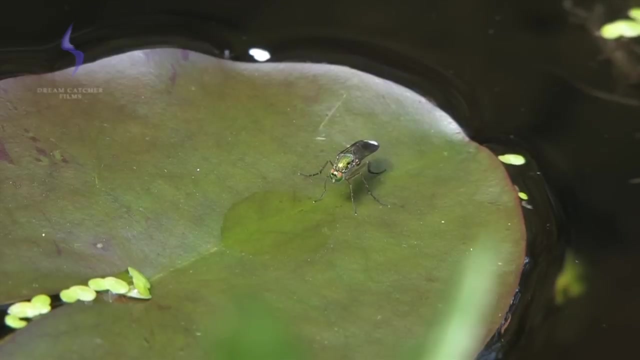 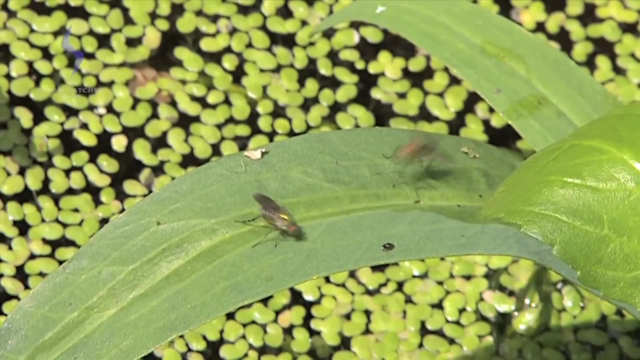 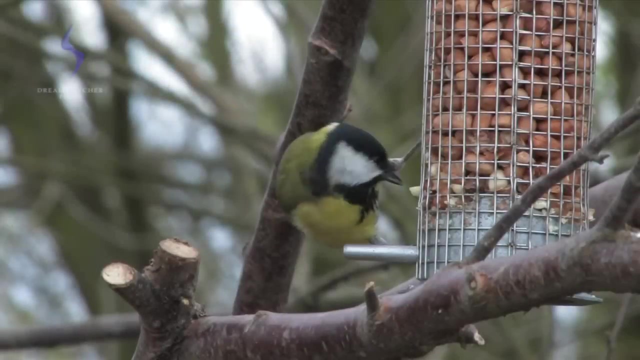 competition. this normally involves the males of certain species that are more abhorrent companions and those who control growth over time. the most common type of feline flying is a collective top llev Rodson el bansem in the ew ce p resurrected bay for a breath in this viewingIDE. agents and species displaying 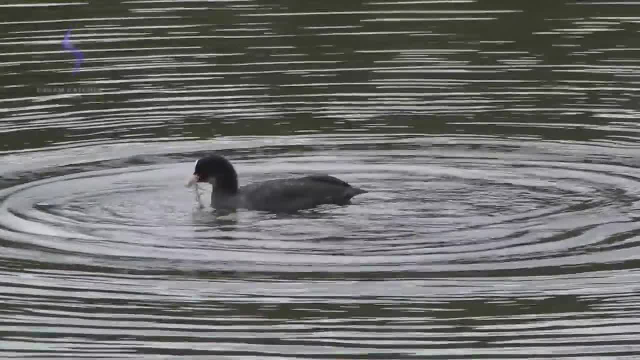 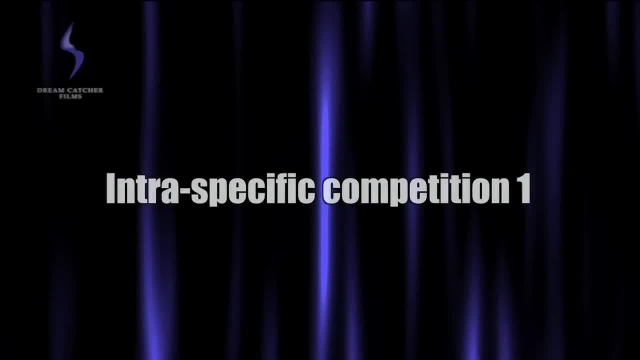 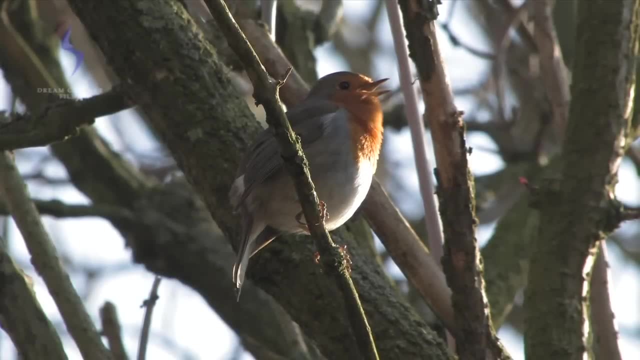 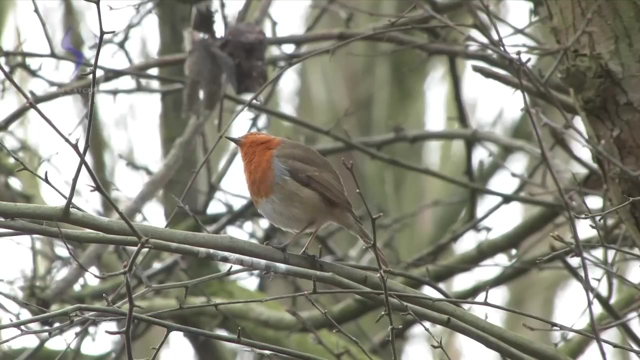 population growth rate will be affected, unless it can be compensated by a reduction in intraspecific competition. what is intraspecific competition? this occurs when two or more individuals of the same species strive for the same resource. this is easily observed, as it often leads to very visual or noisy contests. many species become territorial. 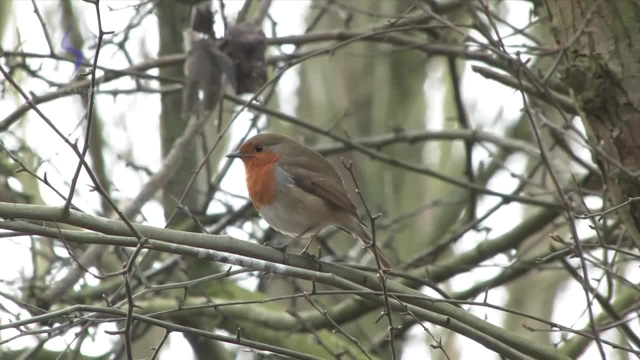 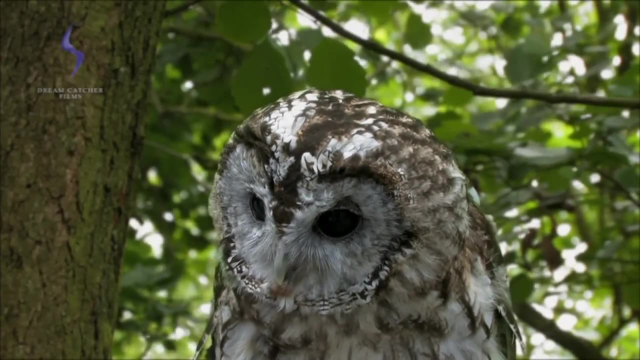 in defense of their species, and in defense of their species and in defense of their valuable food resources. robins are an obvious example of this sort of behavior. birdsong is an audible expression of this contest for resources. similarly, tawny owls are fiercely territorial. they pair for life and defend their breeding. 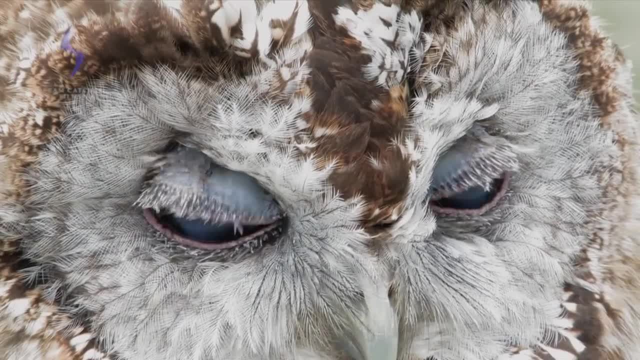 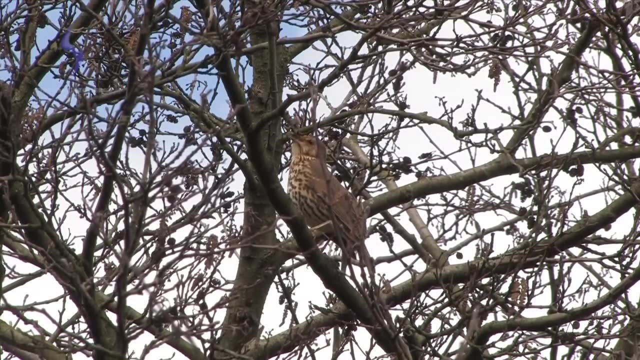 area against all other tawny owls in order to secure the food resources and nesting sites. at the population level, intraspecific competition is a very important factor in the survival of the species and the survival of the species. intraspecific competition for resources can bring about the overall decline in. 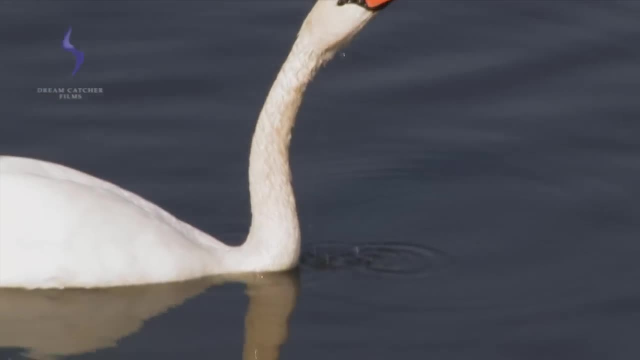 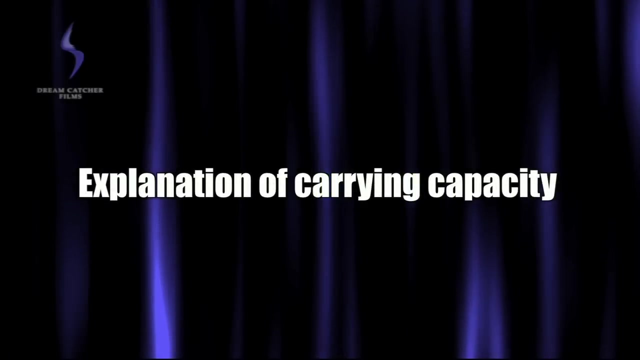 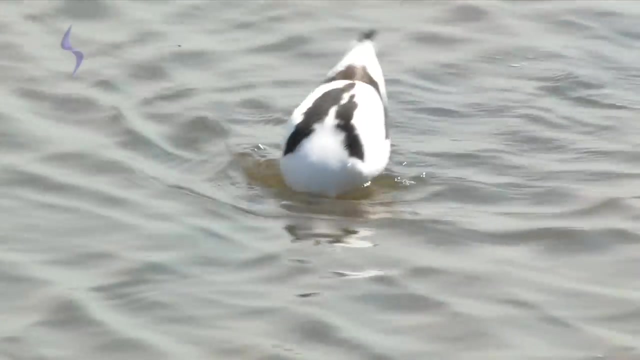 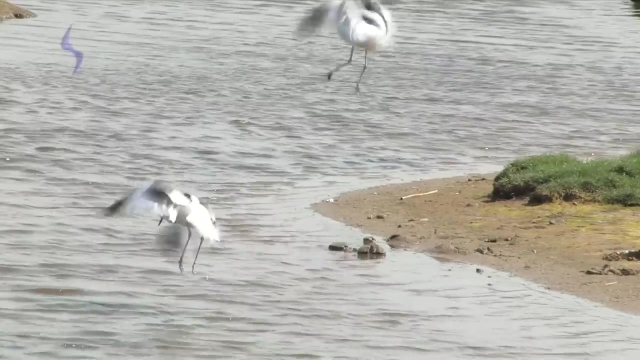 population of an organism when it exceeds the carrying capacity of its environment. carrying capacity is defined as the maximum number of individuals of a given species that a site can support during the most unfavorable time of year without causing deterioration of the site. this is what would determine the maximum number of avocets that can be. 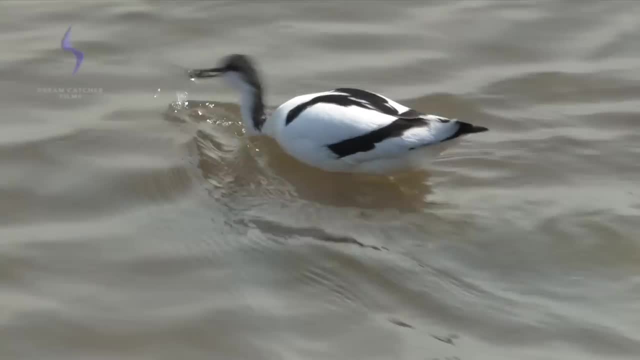 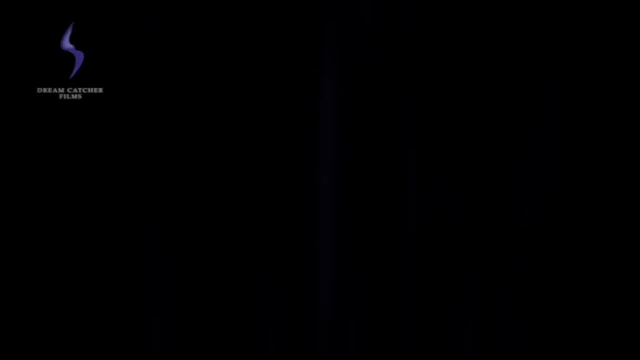 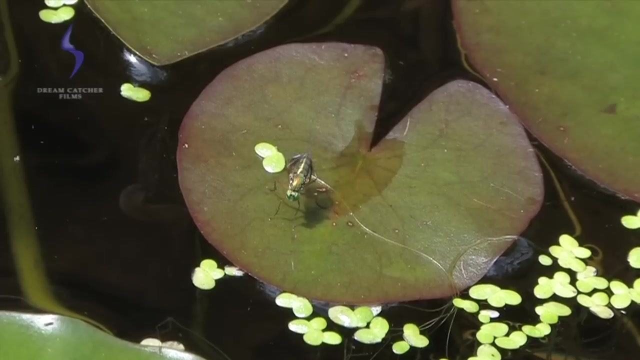 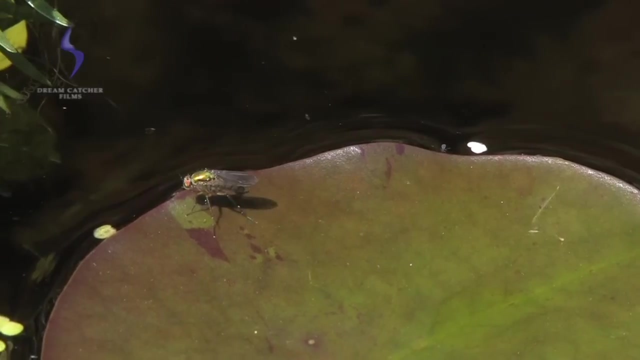 supported on breeding lagoons, feeding on small aquatic invertebrates without reducing their ability to find enough food to sustain them. lecking is one of the more extreme examples of visible intraspecific competition. this normally involves the males of certain species, such as the. 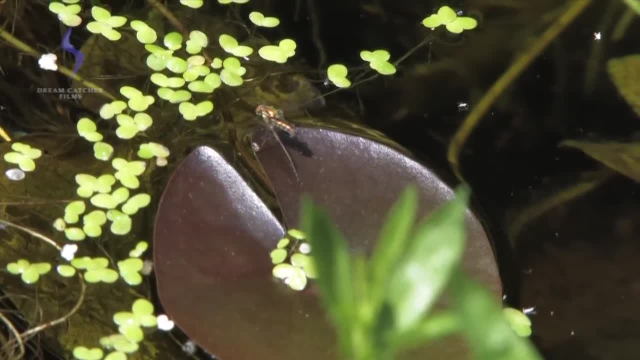 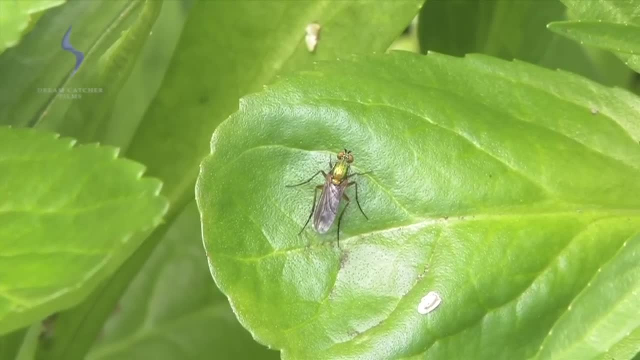 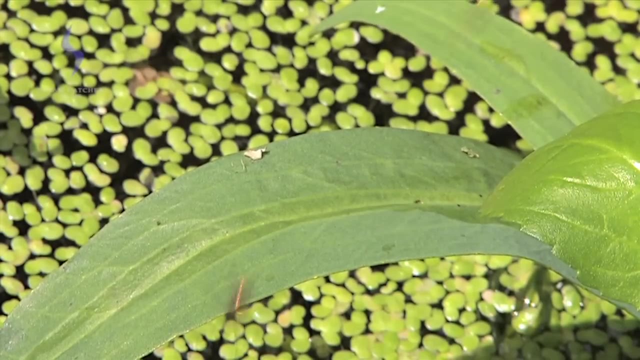 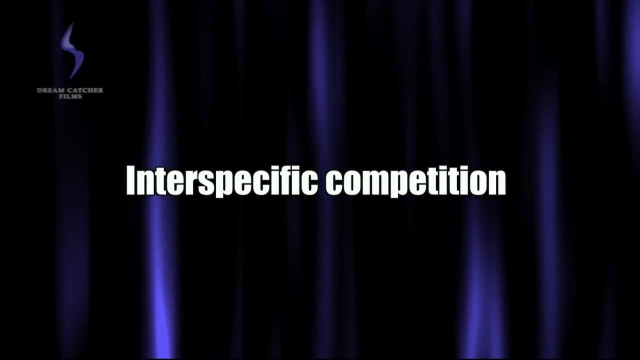 common species display in on a communal lecking ground. these male dance flies for melec and compete for the attention of visiting females. they flirt their decorated wings in the hope of enticing the females to mate and also to intimidate the rival males. you birds on feeders. demonstrating their ability to have food and feed on the same day is also evident in flying otters. as in the Major League League of laws. on a communal 역. in ground, these male danceflies form a lack and compete for the attention of visiting females. they flirt their decorated wings in the hope of enticing the females to mate and also to intimidate the rival males. now long himmek is in the United States. 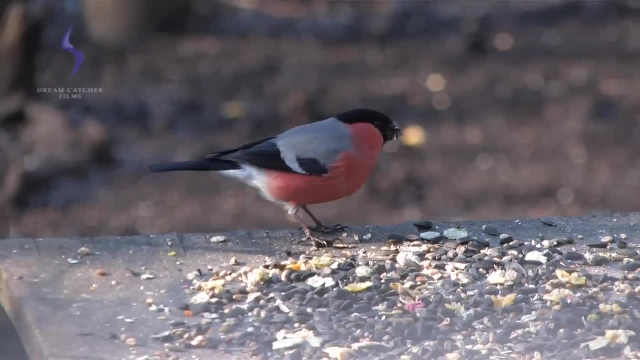 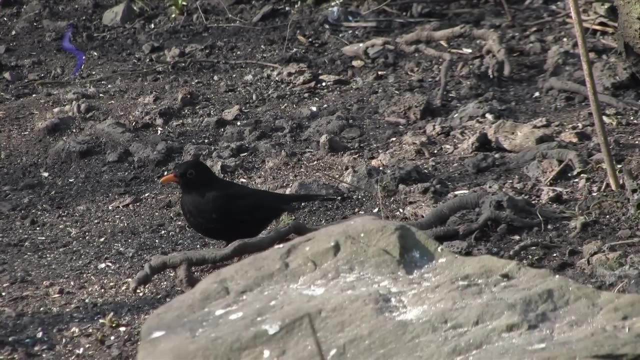 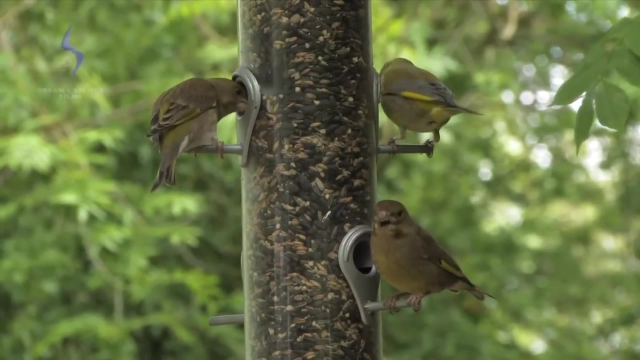 on feeders demonstrate a dominance hierarchy between species. This is an example of interspecific competition. In ecology, this is a form of competition in which individuals of different species vie for the same resource. in an ecosystem, Interspecific competition is a powerful driving force for evolution. 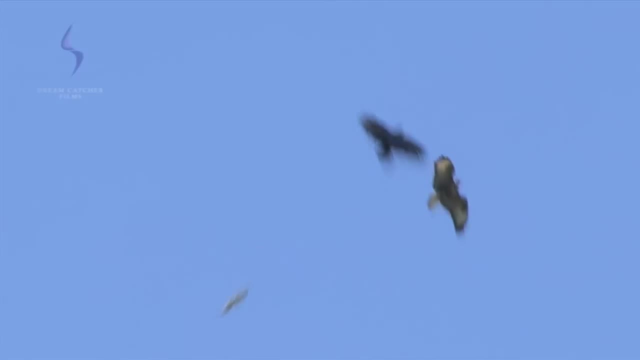 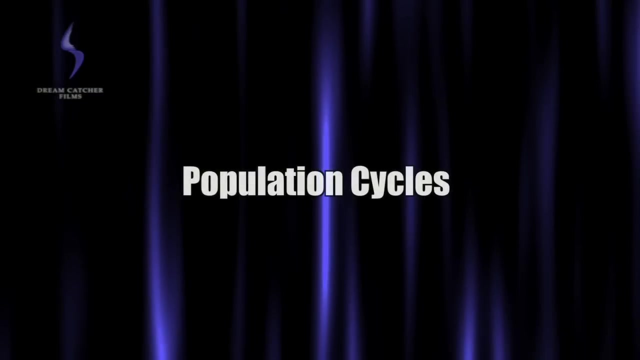 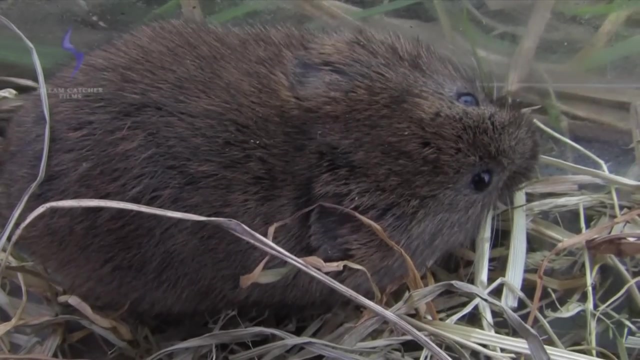 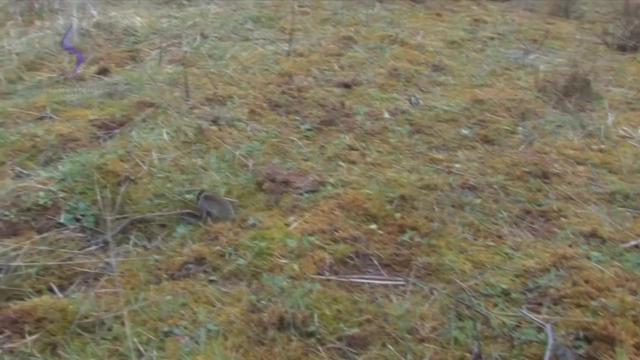 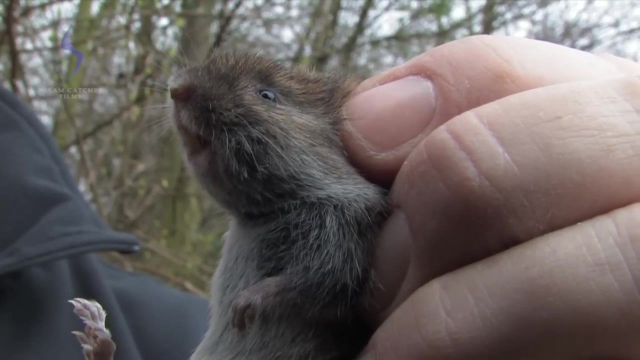 Most species avoid this sort of competition by targeting different food resources or exploiting them in different ways. Intraspecific competition in field voles creates cyclical booms and busts in the population. During the boom phase, the population density in a given area increases dramatically. However, there comes a point when there are too many. 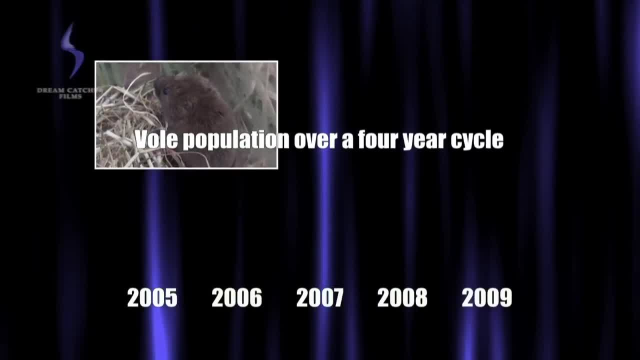 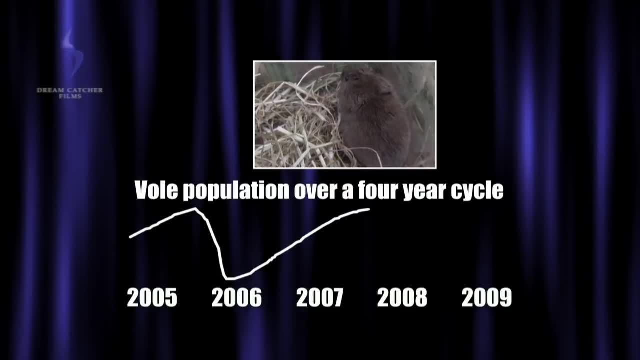 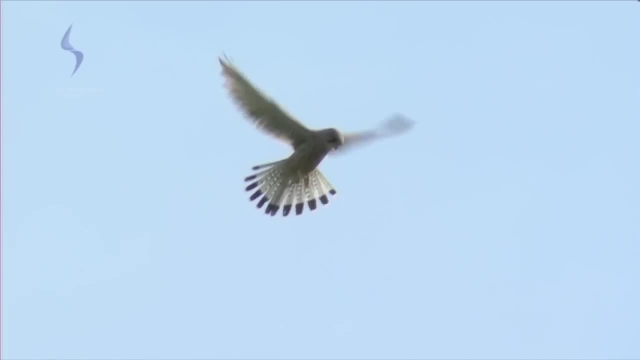 voles and not enough food. There then follows a dramatic die-off and the numbers of voles crash. Most vole populations undergo these crashes on a three or four year cycle. In the voles boom phase, kestrels do very well and raise many young In the year following a. 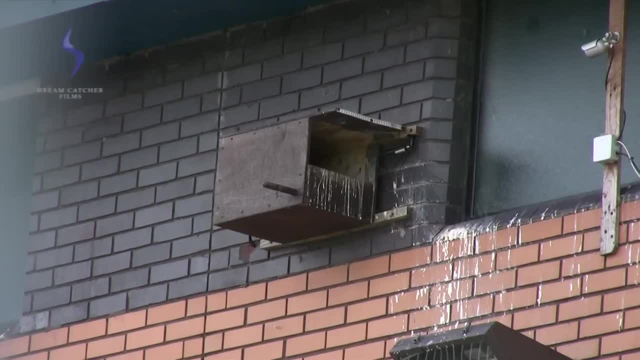 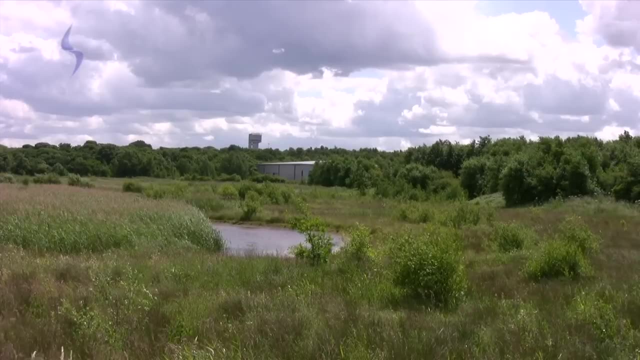 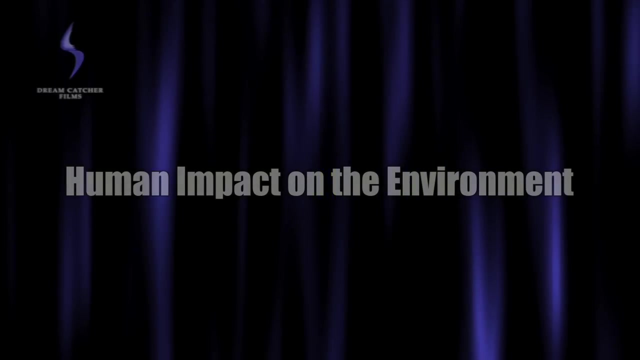 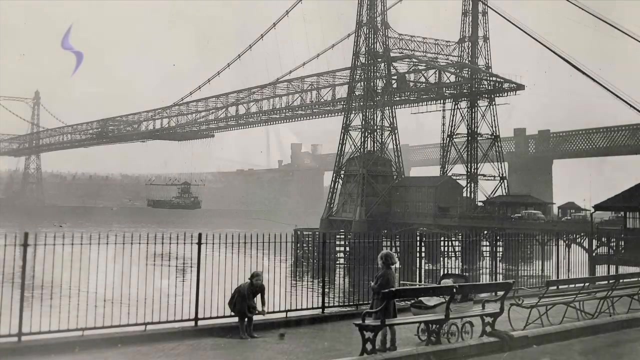 crash. there may be so few voles around that kestrels don't even breed, and in the worst years, many kestrels move out of an area in search of better food resources Or die of starvation. The actions of humankind have had, and continue to have, a profound impact on 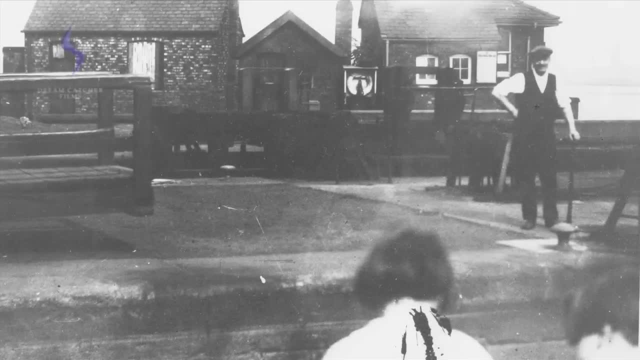 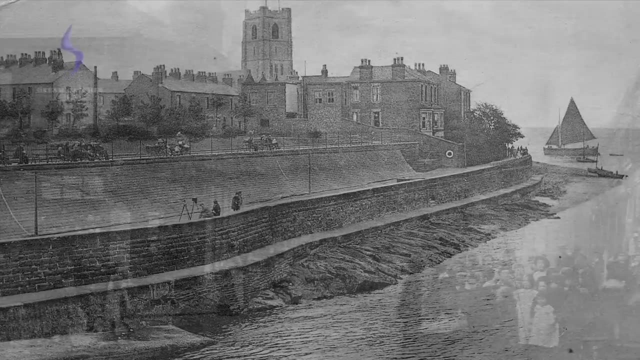 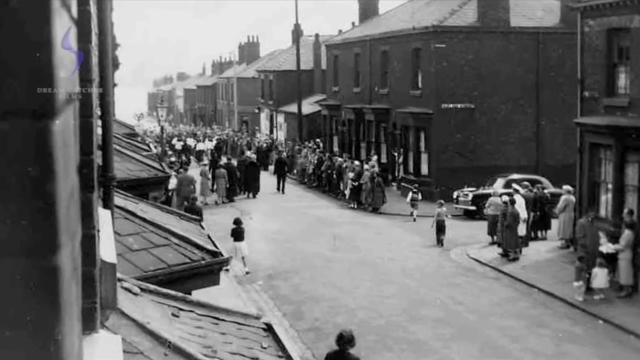 the natural environment, even to the point of tipping the balance in predator and prey relationships. This is West Bank in Widnes, an area that was so ravaged by industrial pollution at the turn of the 19th and 20th century that the average life expectancy of its residents was a mere 47 years. 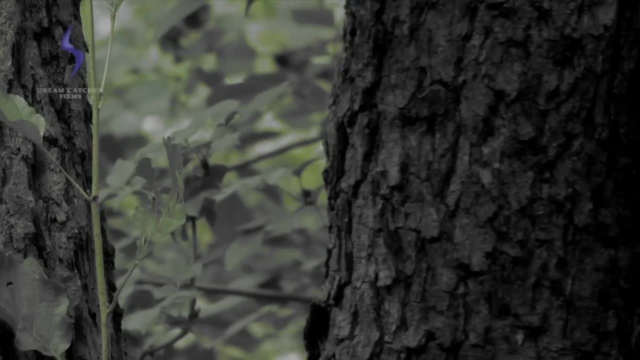 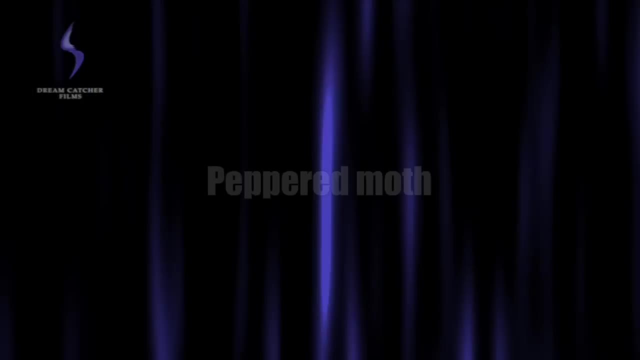 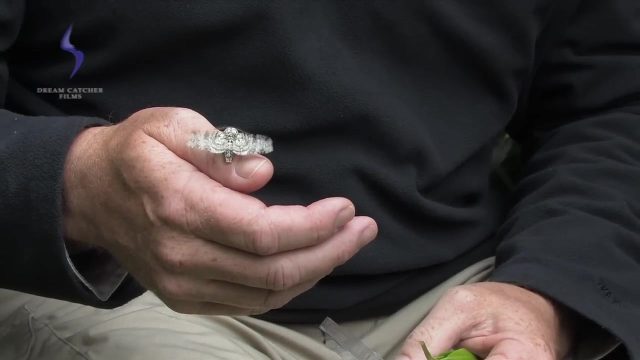 The pollution was so insidious that any trees that survived were covered in black soot and no trace of lichen or moss could grow on the bark. In terms of the study of population dynamics, this creature, the peppered moth, is one of the most important. 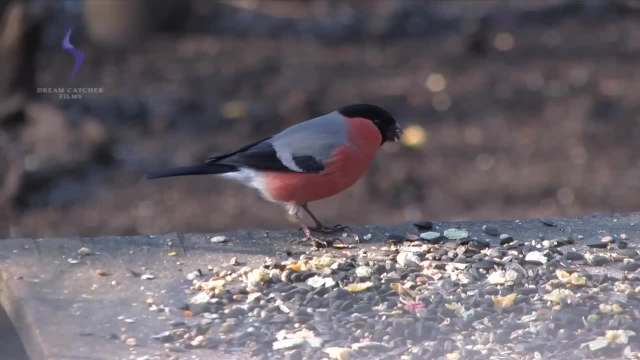 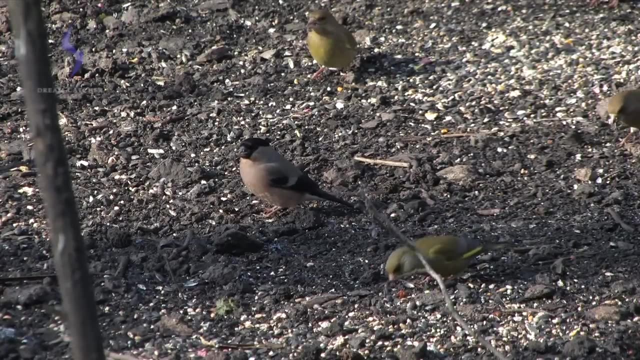 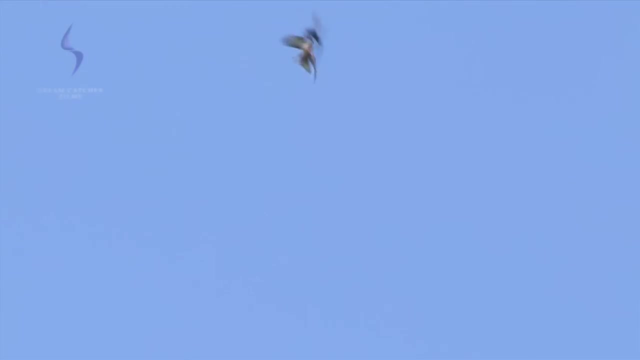 a dominance hierarchy between species. this is an example of inter-specific competition. in ecology, this is a form of competition in which individuals of different species vie for the same resource. in an ecosystem, inter-specific competition is a powerful driving force for evolution. most species avoid this sort of competition by targeting different food resources. 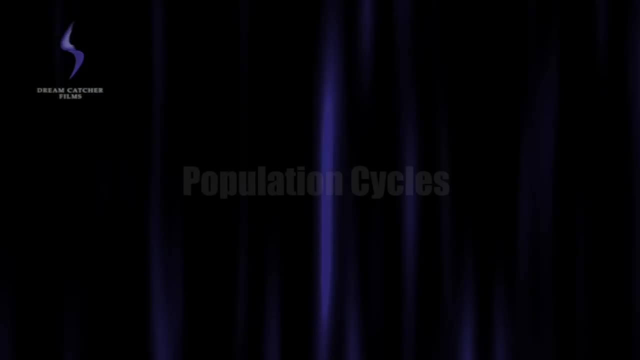 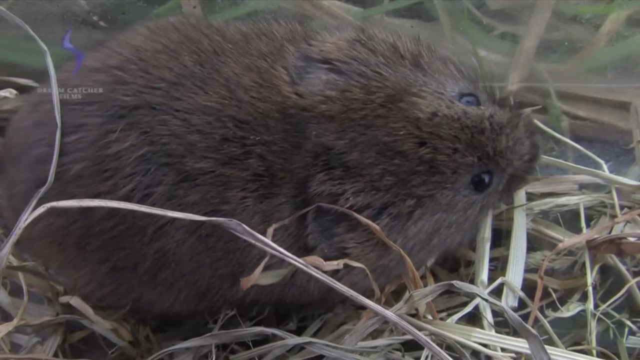 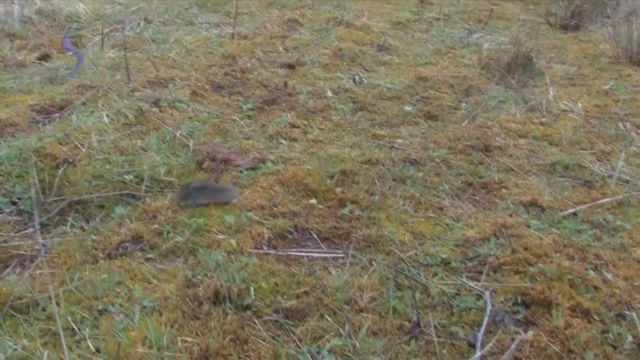 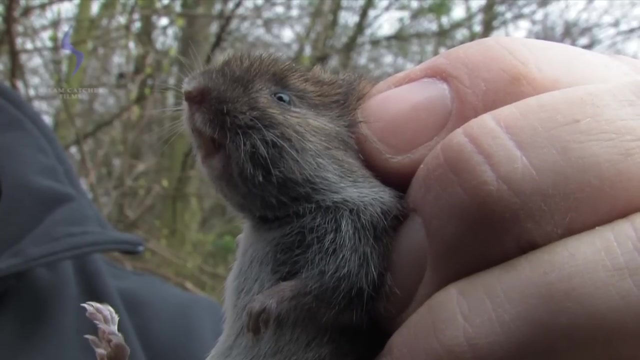 or exploiting them in different ways. intra-specific competition in field voles creates cyclical booms and busts in the population. during the boom phase, the population density in a given area increases dramatically. however, there comes a point when there are too many voles and not enough food. 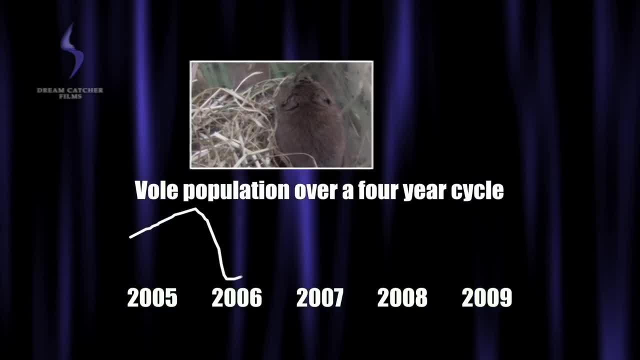 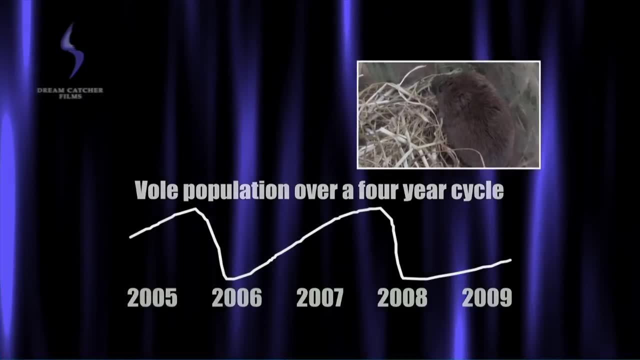 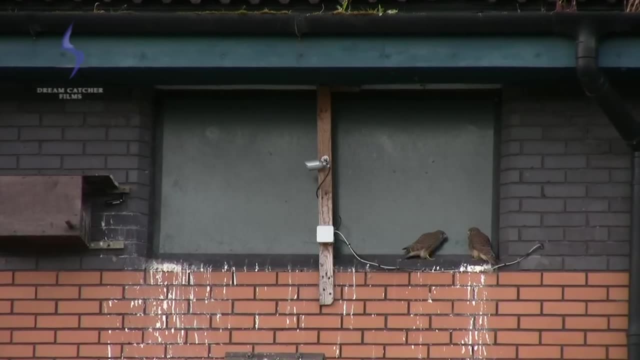 there then follows a dramatic die-off and the numbers of voles crash. most vole populations undergo these crashes on a three or four year cycle. in the voles boom phase, kestrels do very well and raise many young. in the year following a crash there may be so few voles around that kestrels don't even breed. 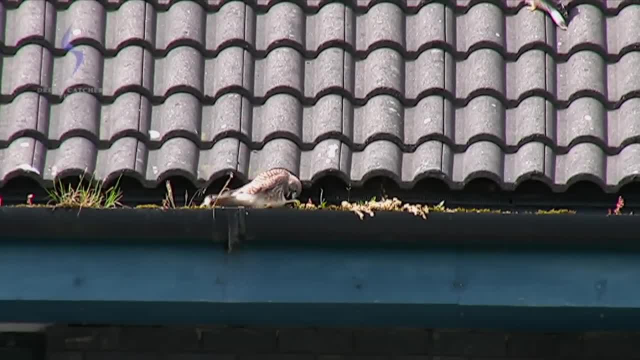 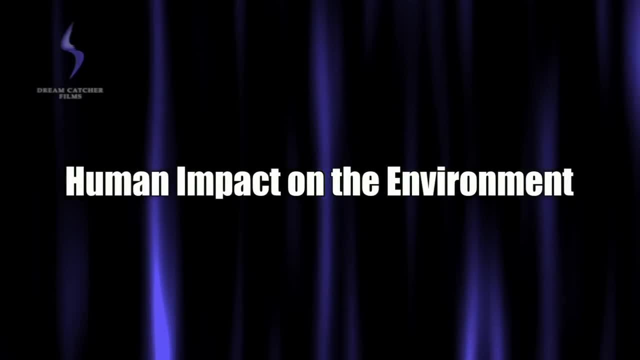 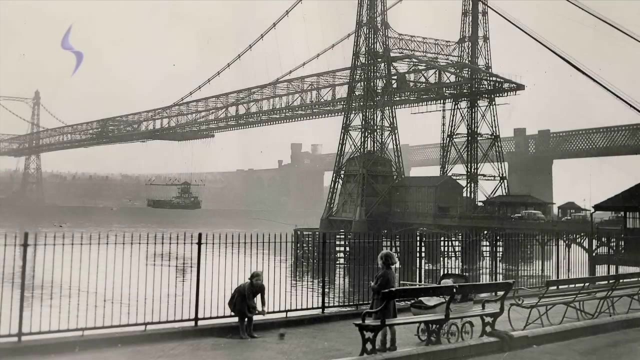 and in the worst years, many kestrels move out of an area in search of better food resources, and the most often they die in the year following a crash. the most common cause of death is starvation. the actions of humankind have had, and continue to have, a profound impact on the natural environment. 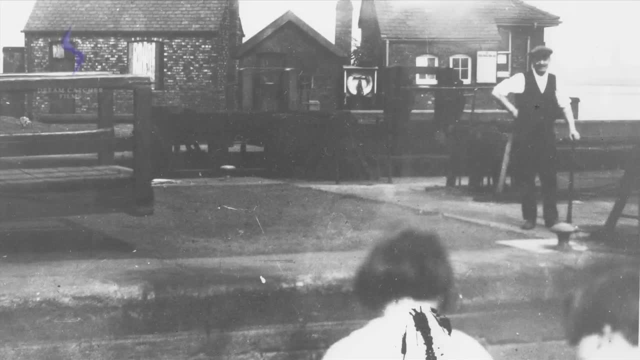 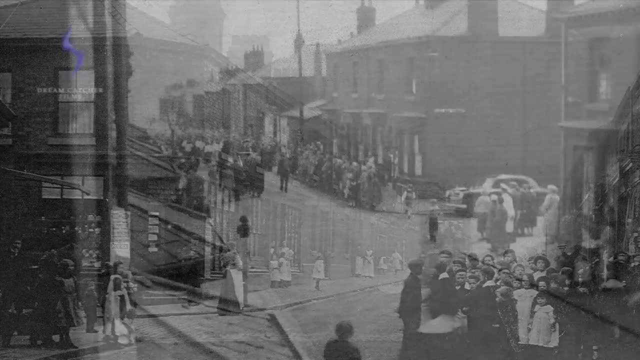 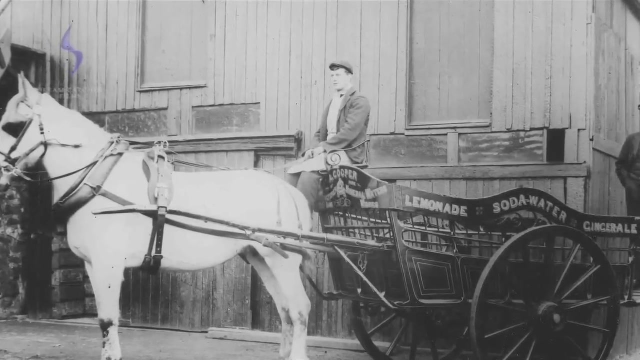 even to the point of tipping the balance in predator and prey relationships. this is west bank in witness, an area that was so ravaged by industrial pollution at the turn of the 19th and 20th century that the average life expectancy of its residents was a mere 47 years. 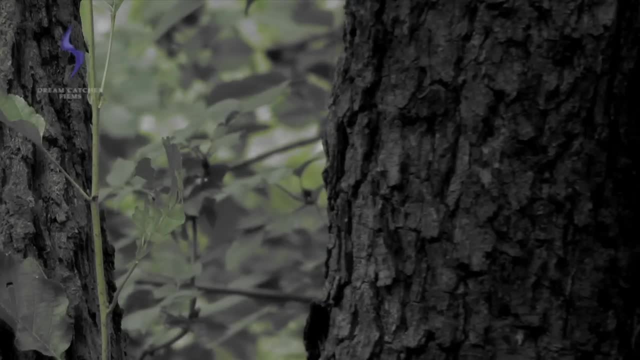 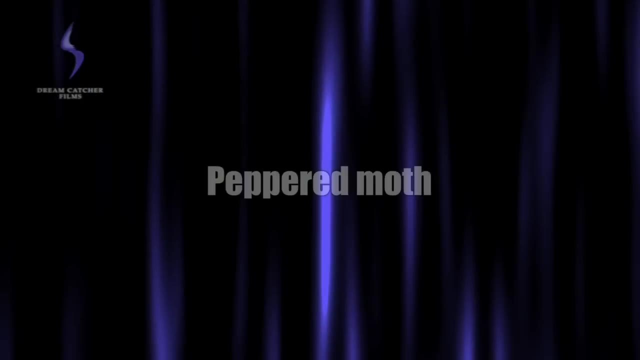 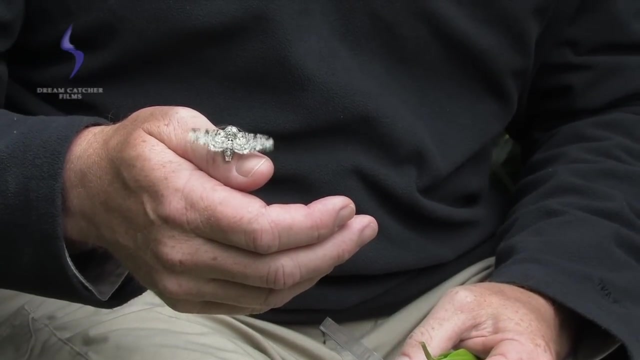 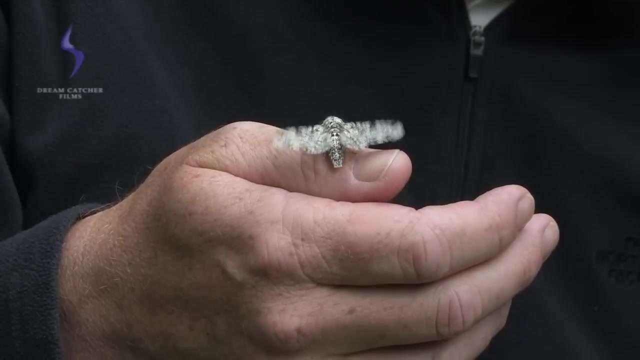 the pollution was so insidious that any trees that survived were covered in black soot and no trace of lichen or moss could grow on the bark. in terms of the study of population dynamics, this creature, the peppered moth, is one of the most important. the industrial revolution created changes which forced this creature to adopt a 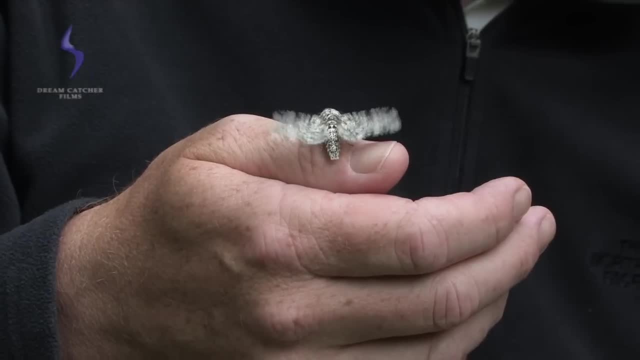 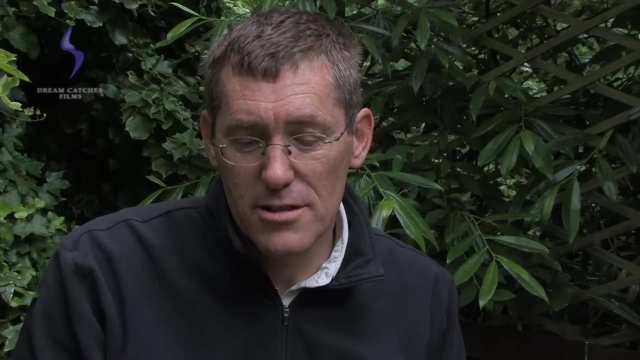 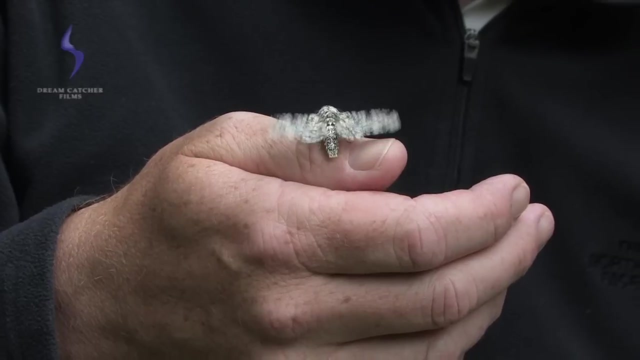 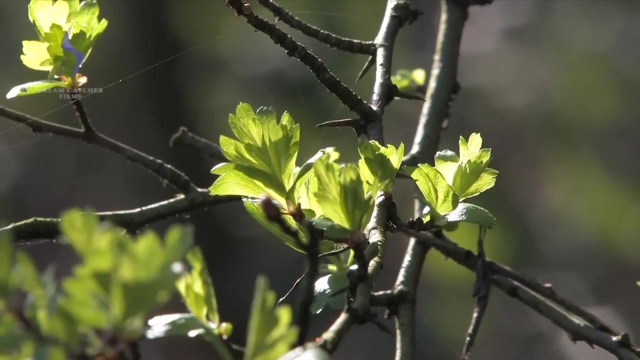 The industrial revolution created changes which forced this creature to adopt a different colour form, a black form. Today in Halton they're virtually all back in this peppered form, and that's the change that's been brought about by the Clean Air Act. Some invertebrate species were able to cope with that pollution because they only fed upon the annual flush of leaves. 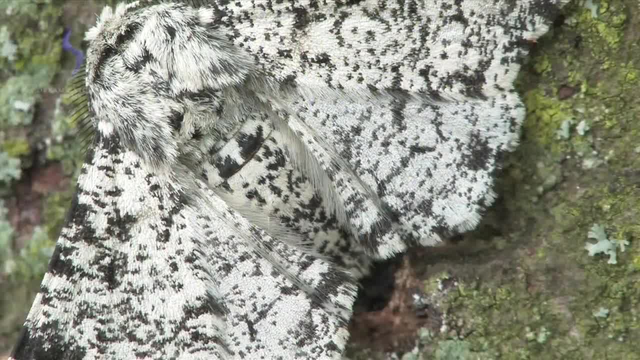 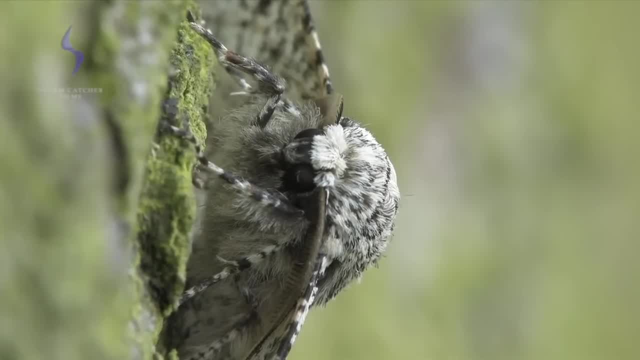 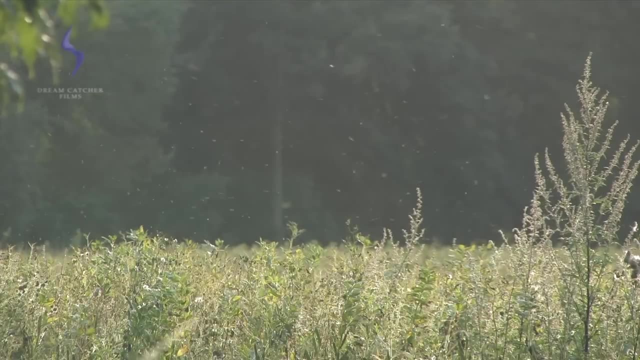 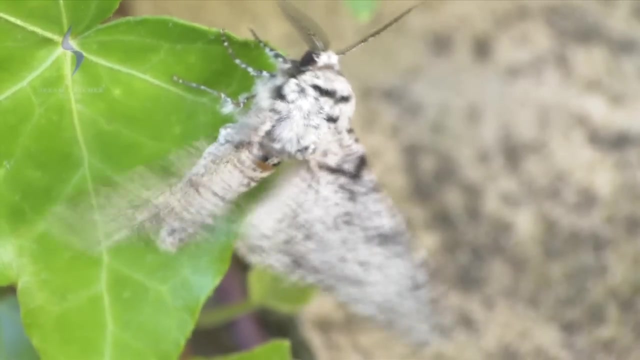 One such species was the peppered moth. This attractively marked moth is one of the most important pieces of evidence we have in our understanding of both evolutionary processes and predator-prey relationships. Prior to the industrial revolution, all peppered moths were like this: white with a liberal sprinkling of black spots. 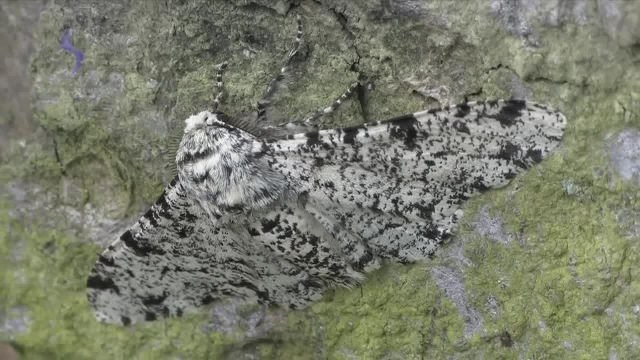 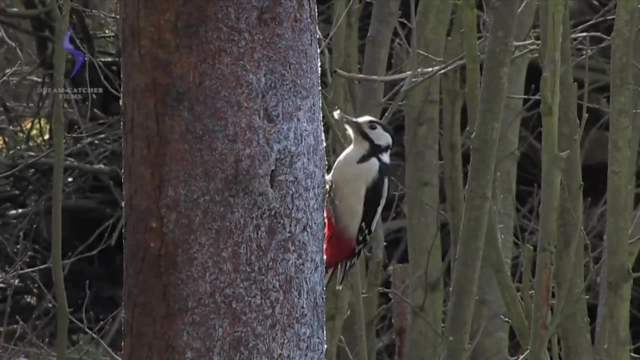 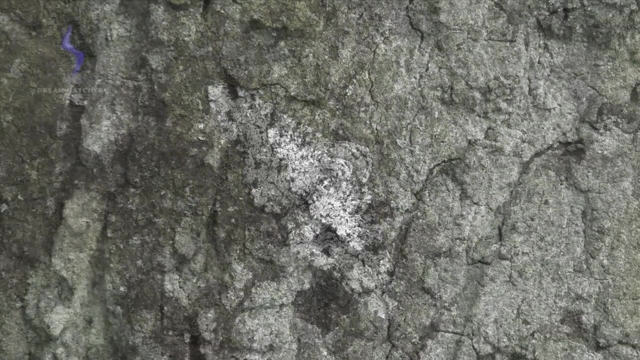 This afforded excellent camouflage protection on the lichen-covered branches, where it rested by day and helped to hide it from predatory birds like the great spotted woodpecker. The soot-covered trees of the 19th century meant that these moths suddenly stood out like a sore thumb. 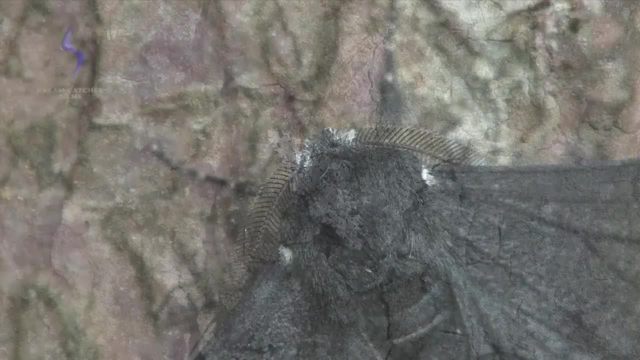 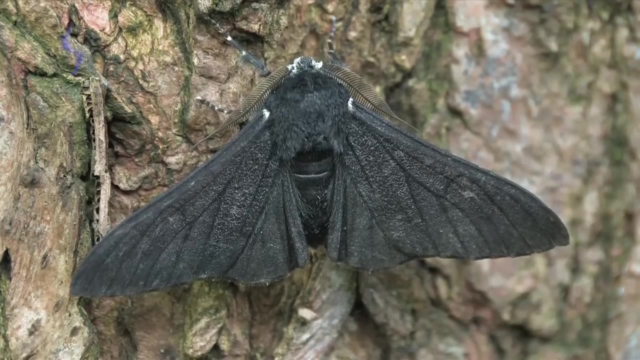 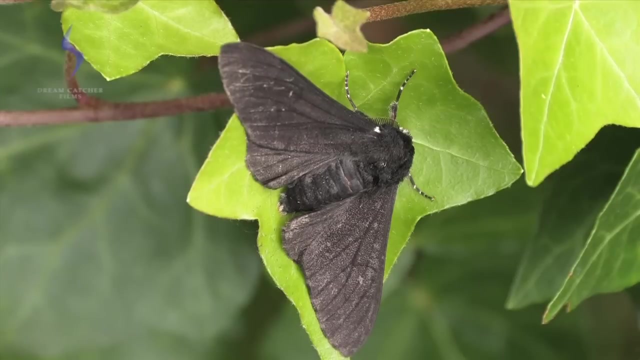 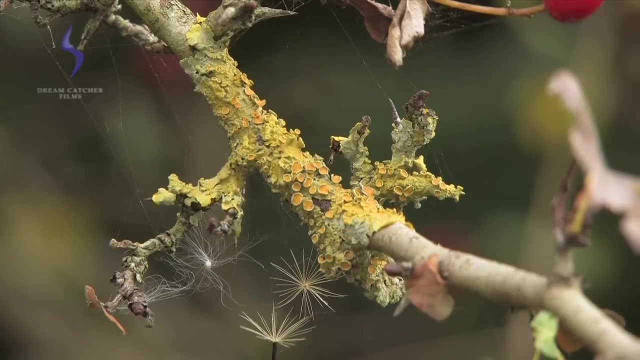 making them more vulnerable to predation. Fortunately for the peppered moth, a chance genetic mutation allowed this black form to evolve Within a few short years. almost 100% of peppered moths in Halton were of the black form. Today, thanks to the huge reductions in atmospheric pollutants, lichens have returned to the trees. 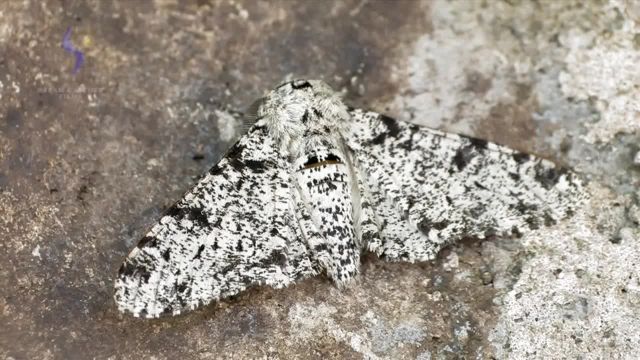 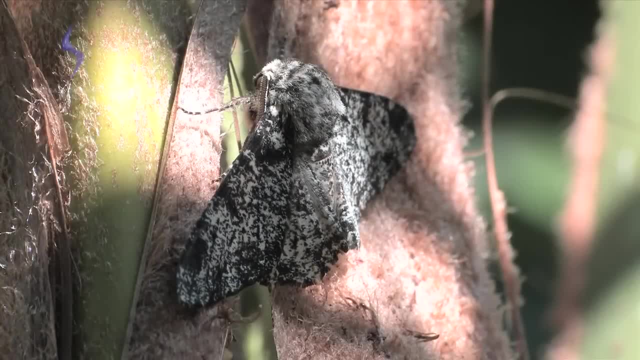 of Halton, and the peppered form is once again the one best hidden from predators. The black form and this partly melanistic form is now very rare, a perfect indicator of the massive improvements that have taken place in Halton's environment. 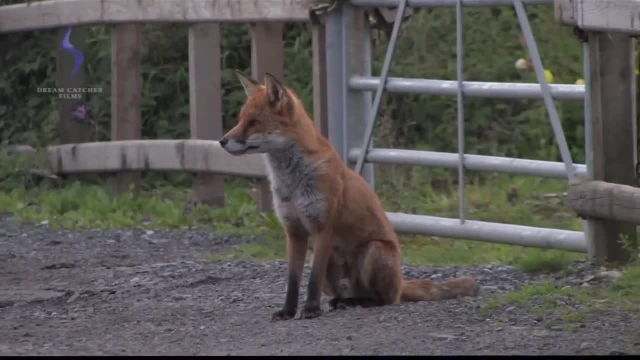 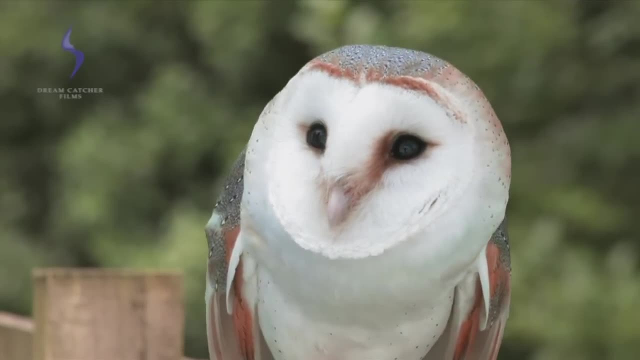 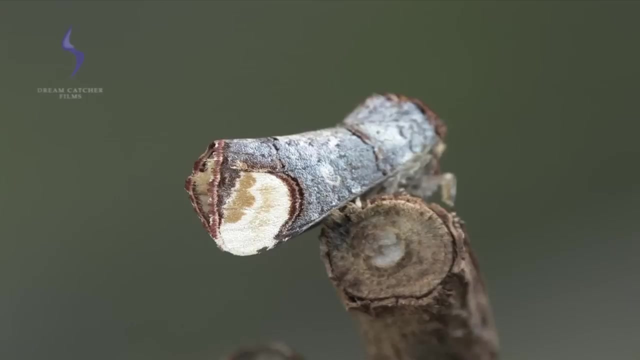 Predators and their prey live in a constant evolutionary arms race. Some of this can be seen in the evolutionary extremes evident in some of our commonest moth species. The incredible and exquisite mimicry of the buff titmoth makes it look astonishingly like a broken birchtwig. 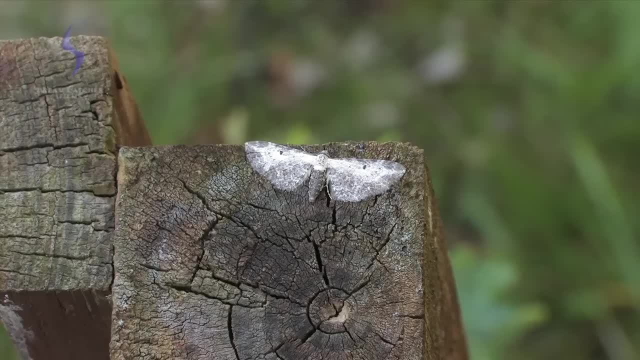 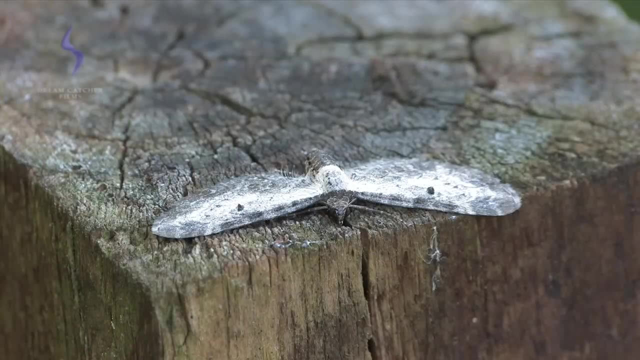 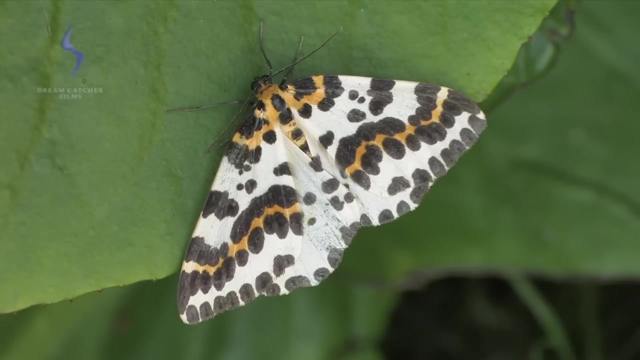 while the bird-poo-mimicking boarded pug creates a different impression in the mind of its predators. Birds know it's there, but don't eat it because it reminds them of something distasteful. This magpie moth wants to be seen and recognised. 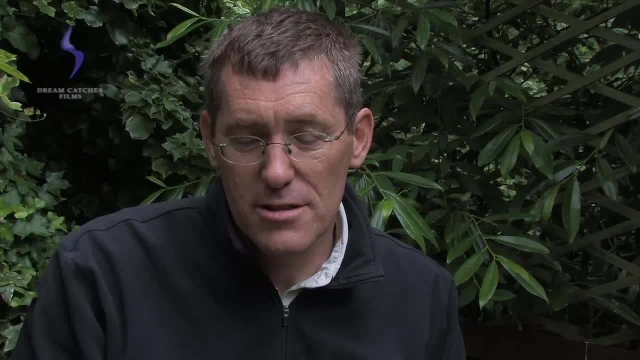 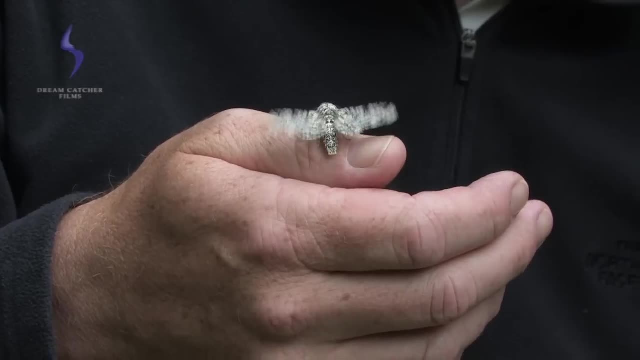 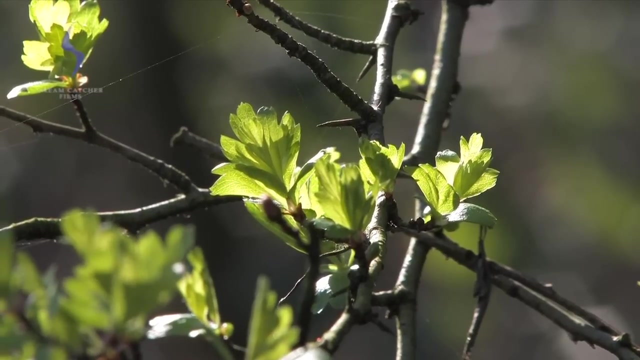 different color form, a black form. today in halton they're virtually all back in this peppered form, and that's the change that's been brought about by the clean air act. some invertebrate species were able to cope with that pollution because they only fed upon the annual flush of leaves. one such 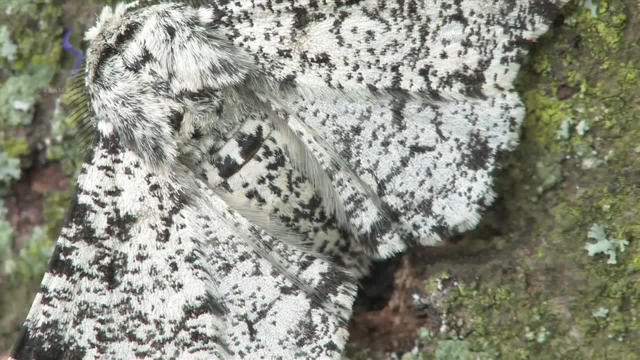 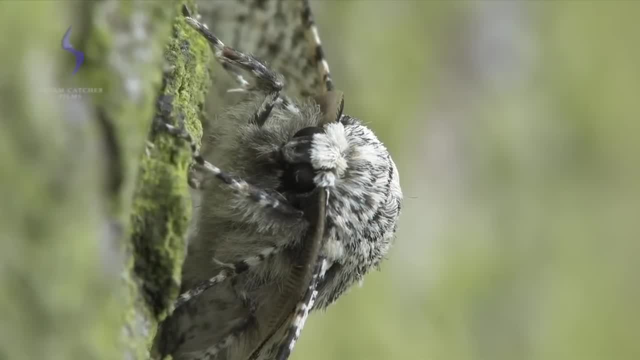 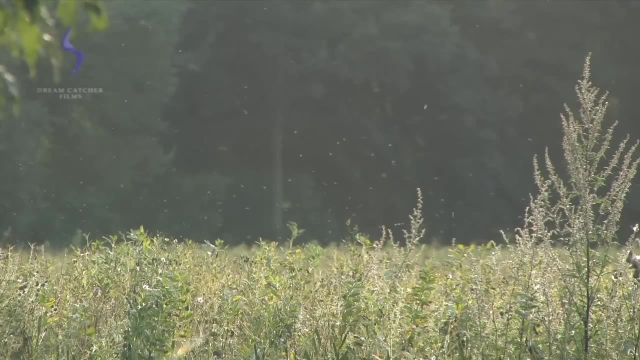 species. was the peppered moth? the peppered moth is one such species. was the peppered moth? this attractively marked moth is one of the most important pieces of evidence we have in our understanding of both evolutionary processes and predator-prey relationships. prior to the industrial revolution, all peppered moths were like this. 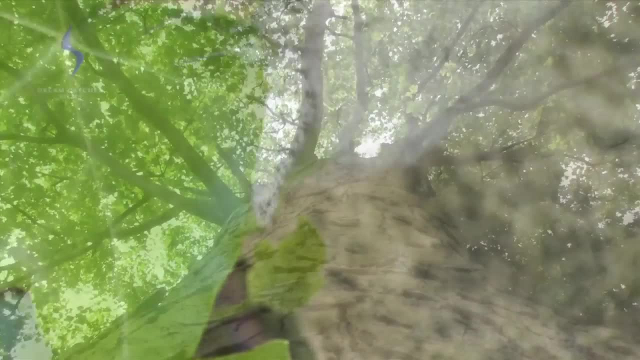 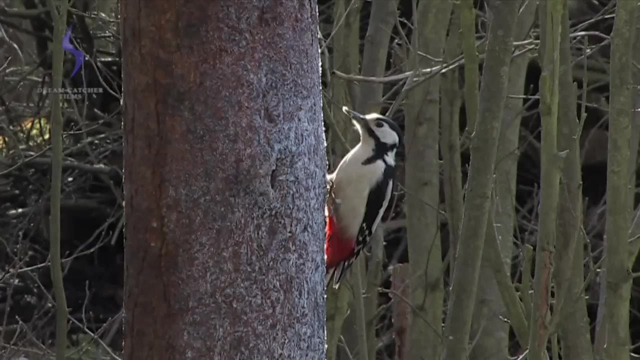 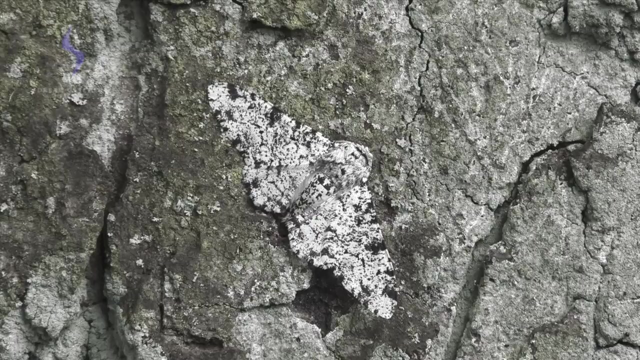 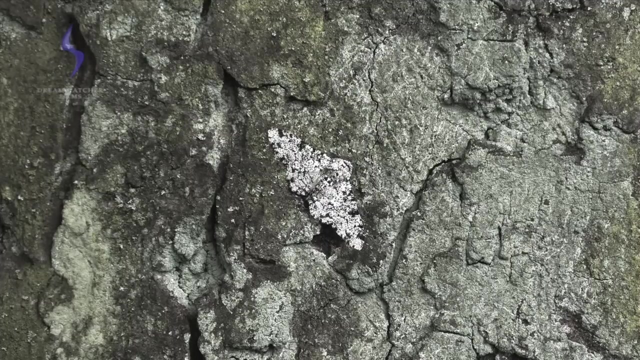 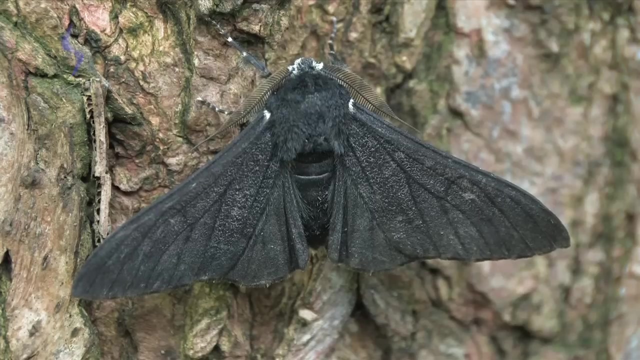 white with a liberal sprinkling of black spots. this afforded excellent camouflage protection on the lichen-covered branches where it rested by day, and the lichen-covered branches were used to protect it from the moths from the wild, and the wild moths were used to protect it from predatory birds like the great. 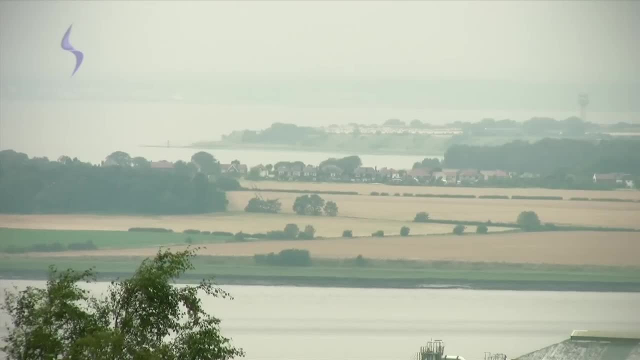 spotted woodpecker. the soot-covered trees of the 19th century meant that these moths suddenly stood out like a sore thumb, making them more vulnerable to predation. fortunately for the peppered moth, a chance genetic mutation allowed this black form to evolve within a few short years. almost 100 percent of peppered moths in halton were of the black form. 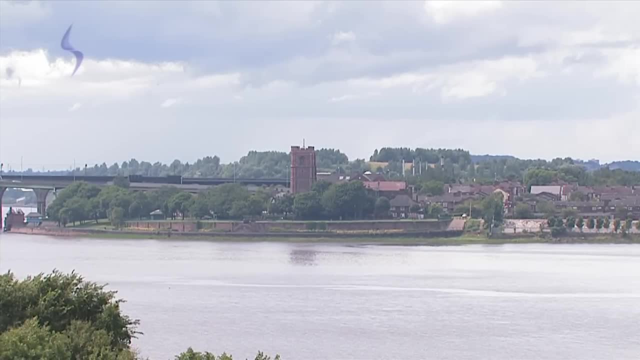 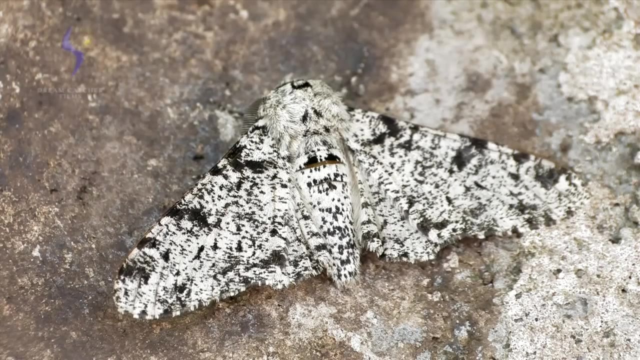 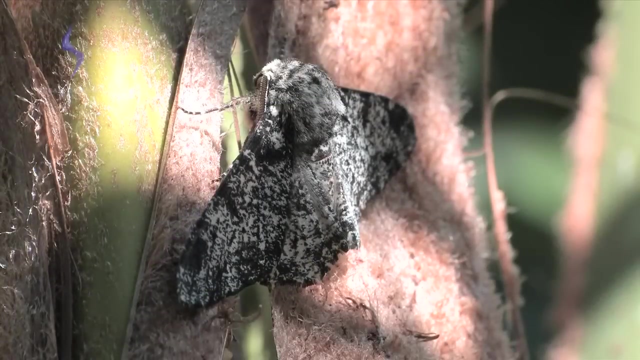 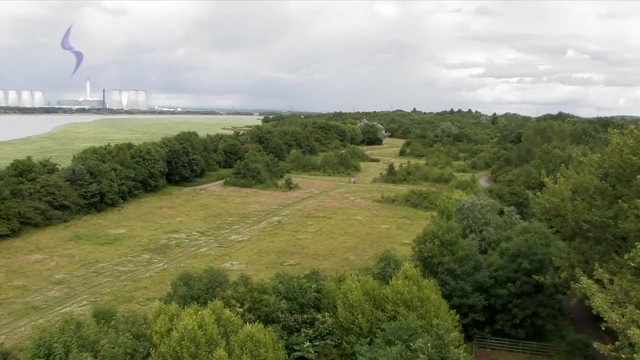 today, thanks to the huge reductions in atmospheric pollutants, lichens have returned to the trees of halton and the peppered form is once again the one best hidden from predators. the black form and this partly melanistic form is now very rare, a perfect indicator of the massive improvements that have taken place in halton's environment. 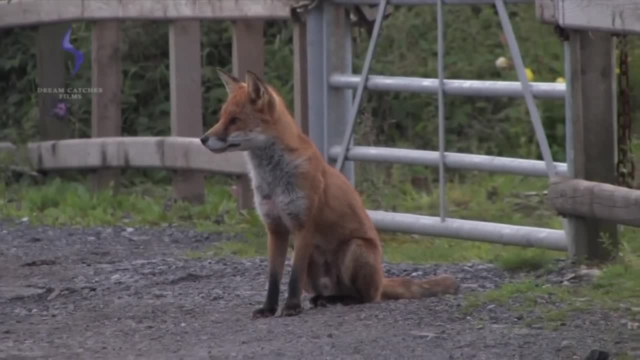 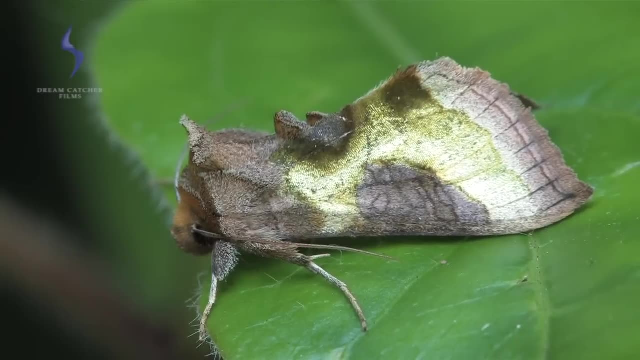 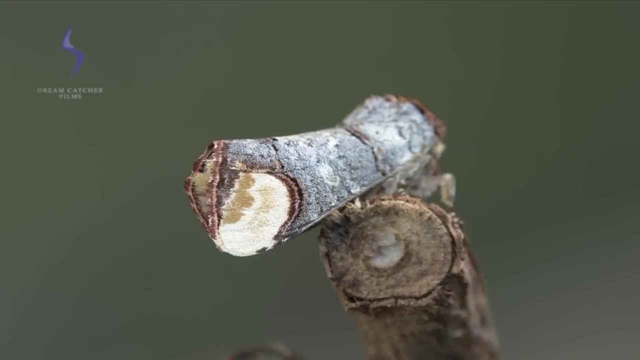 predators and their prey live in a constant evolutionary arms race. some of this can be seen in the evolutionary extremes evident in some of our commonest moth species. the incredible and exquisite mimicry of the buff tip moth makes it look astonishingly like a broken birch twig. 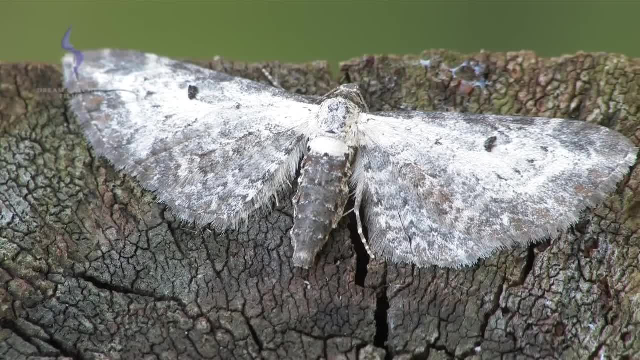 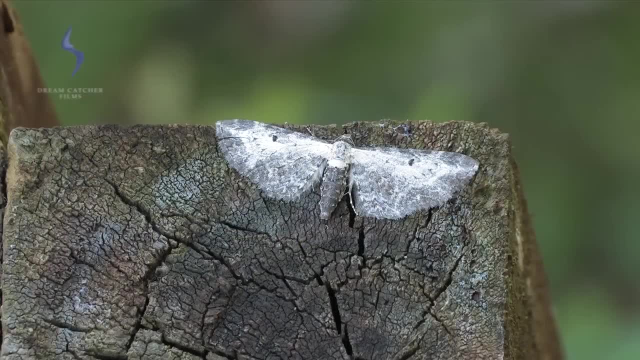 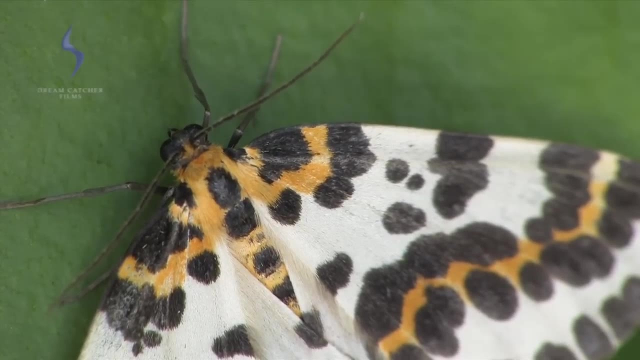 while the bird poo mimicking boarded pug creates a different impression in the mind of its predators. birds know it's there but don't eat it because it reminds them of something distasteful. this magpie moth wants to be seen and recognized. its brilliant markings attract attention telling. 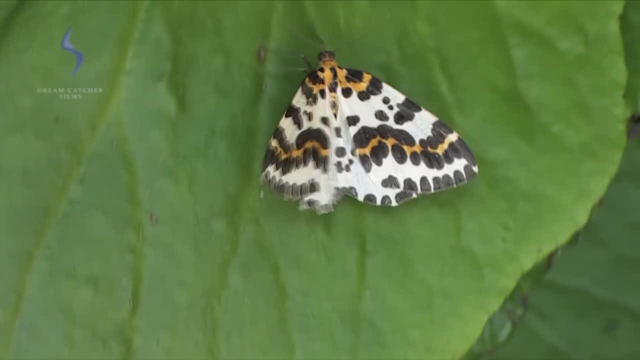 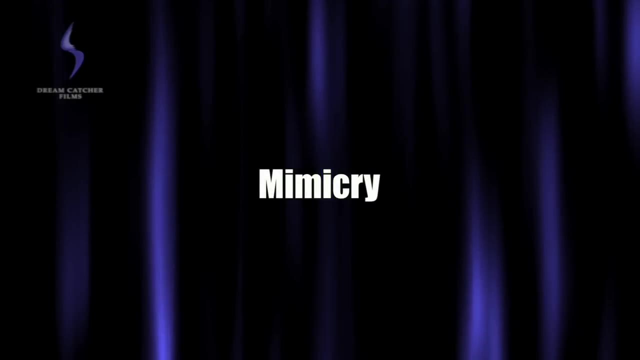 potential bird predators not to bother because it really is loaded with potentially harmful chemical defenses Mr. Givenchy and Her孤 Meng and Mrs. Swanson have � linened her ass two weeks ago just a few weeks ago hurt her family Ну Shadazpabock 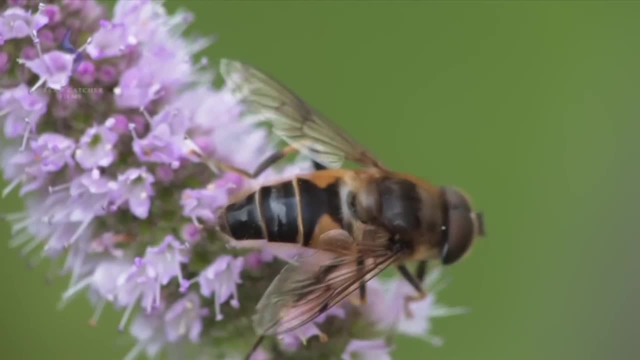 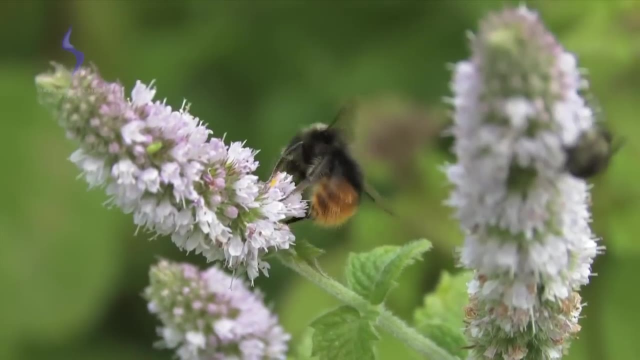 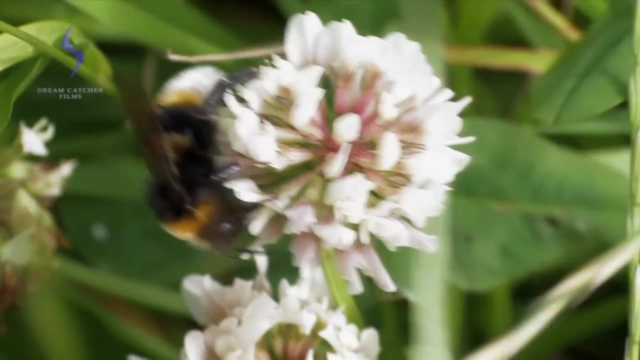 łobysounces found in many species that are familiar to most people. Malarian mimicry involves potentially harmful species, for example wasps and bees, that evolve a common color scheme and pattern to increase the potency of their message. Most potential predators recognize these species as dangerous and leave them alone. 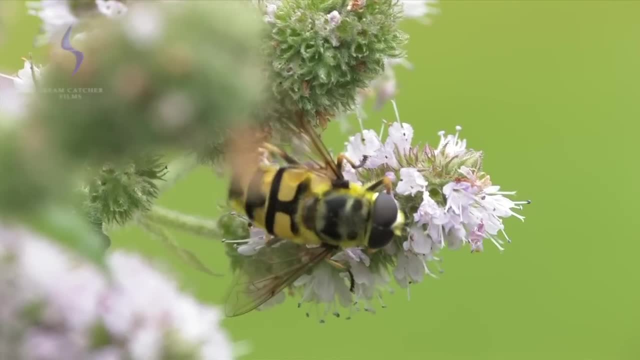 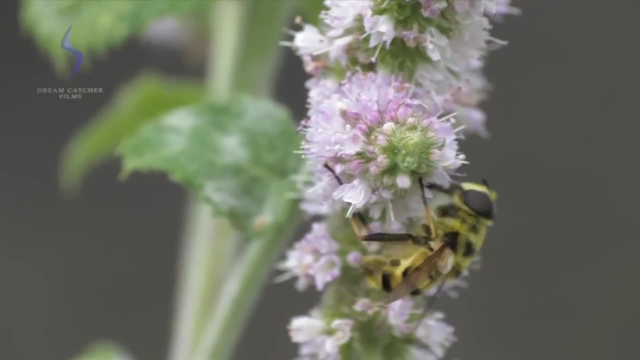 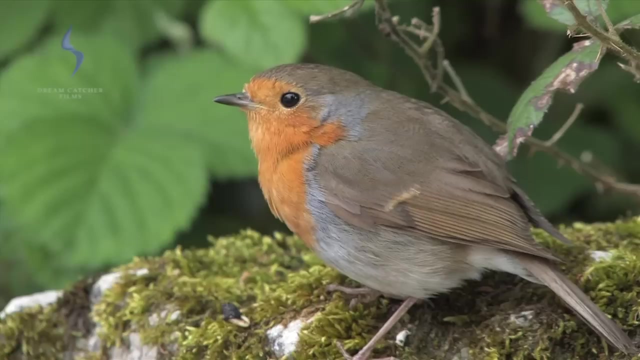 Batesian mimics, like these hoverflies, have evolved colors and patterns that are similar to these well-defended species, and, though they themselves are harmless, they gain a degree of protection from their similarity to the dangerously armed wasps and bees. This does not, however, protect them from some 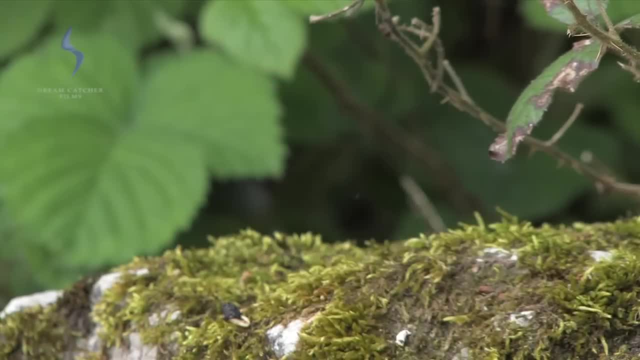 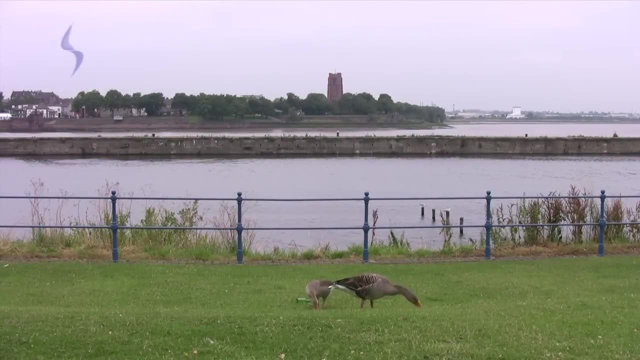 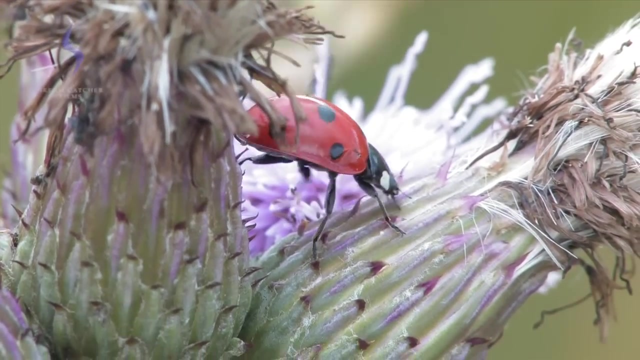 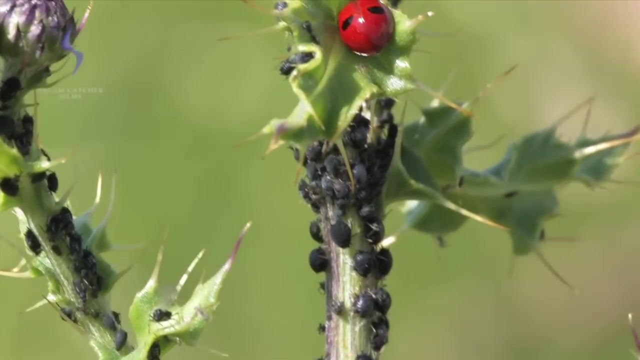 particularly sharp-eyed insect-eating birds. Feeding relationships can be either simple or complex. In a higher form, most predator populations are governed by the availability of prey. Prey levels are rarely limited solely by the impacts of the predator. On the other hand, 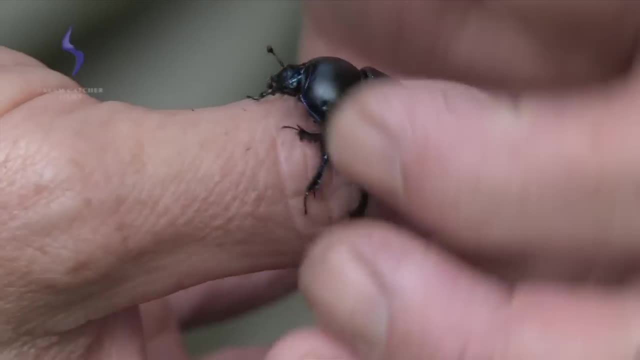 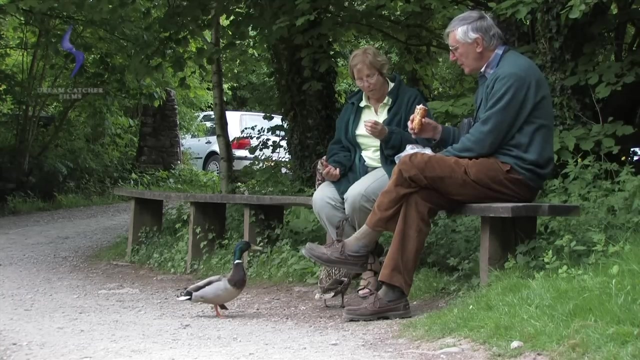 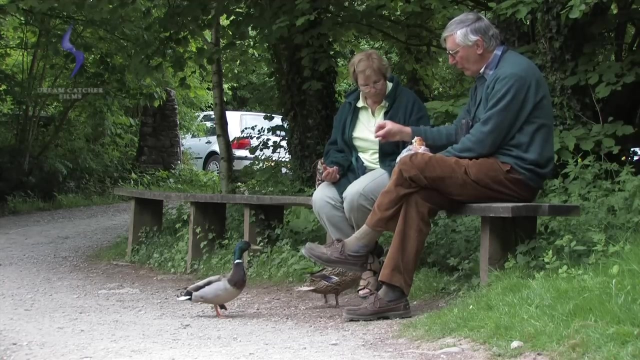 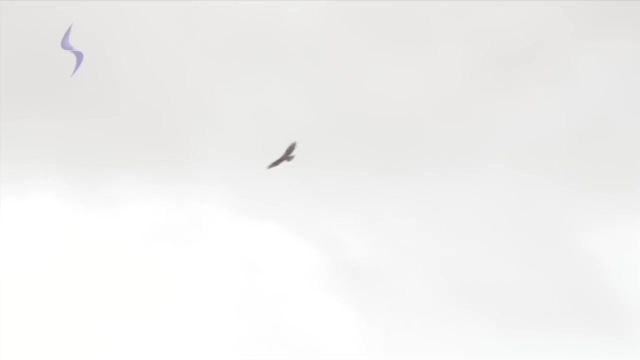 parasitic predation can cause very dramatic declines in the availability of the host species. Except where man introduces an unpredictable variable, most ecosystems maintain a balance of populations And change is normally a slow process. In those circumstances where species undergo dramatic population fluctuations, they normally do so on a predictable cycle. 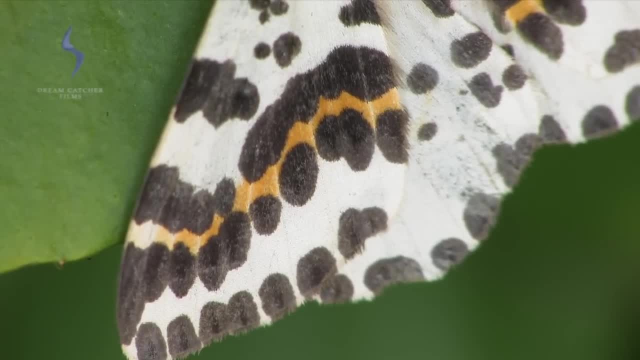 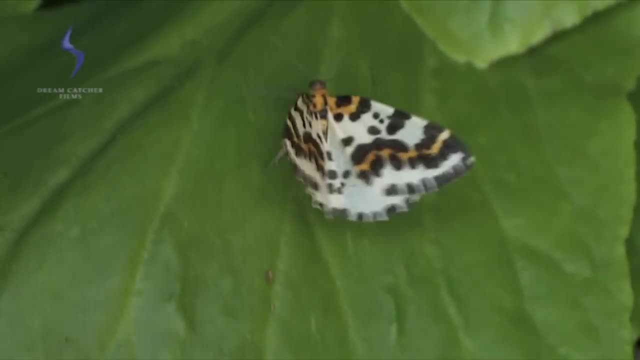 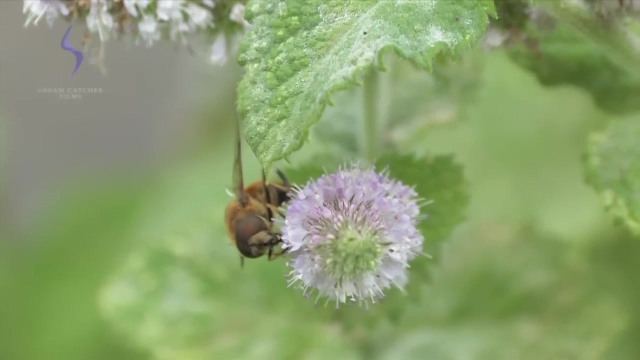 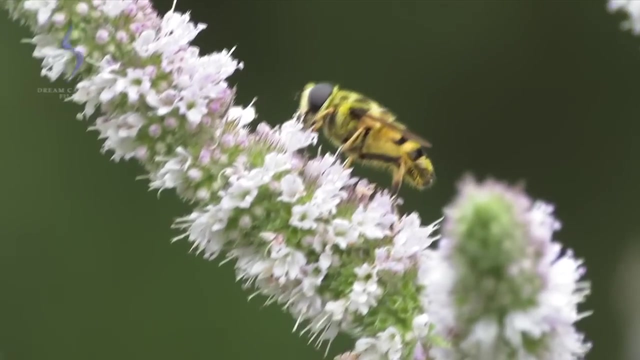 Its brilliant markings attract attention, telling potential bird predators not to bother because it really is loaded with potentially harmful chemical defences. Mimicry Mimicry is commonly found in many species that are familiar to most people. Malarian mimicry involves potentially harmful species, for example wasps and bees. 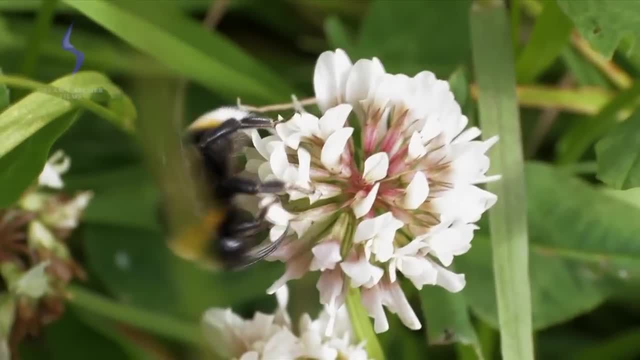 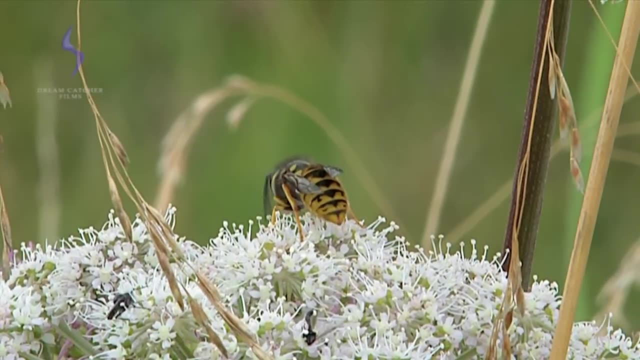 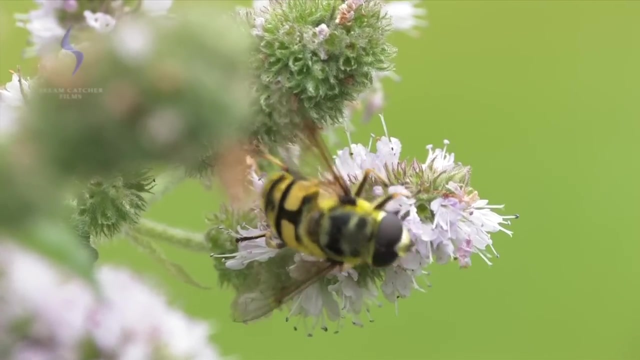 that evolve a common colour scheme and pattern to increase the potency of their message, Most potential predators recognise these species as dangerous and leave them alone. Batesian mimics, like these hoverflies, have evolved colours and patterns that are similar to these well-defended species. 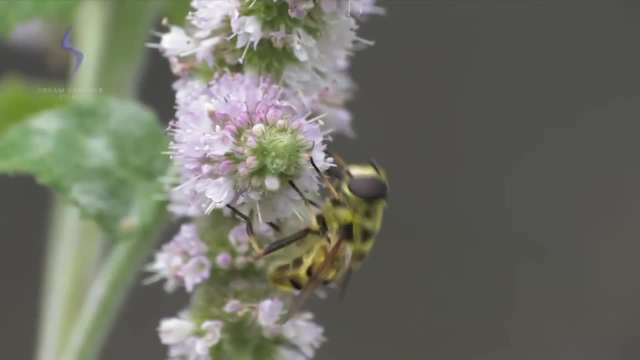 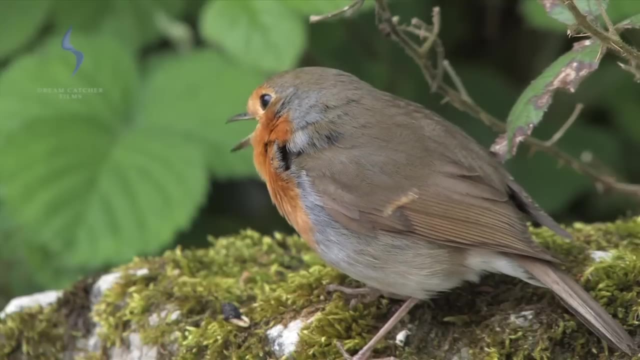 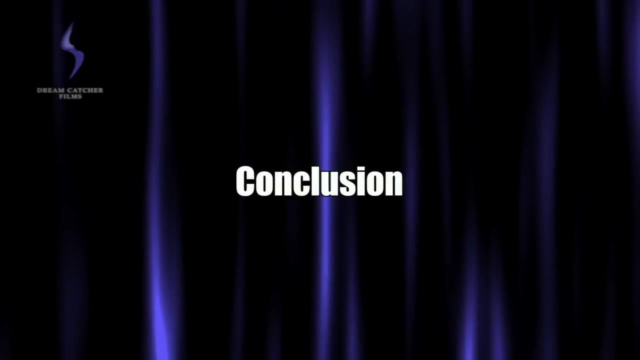 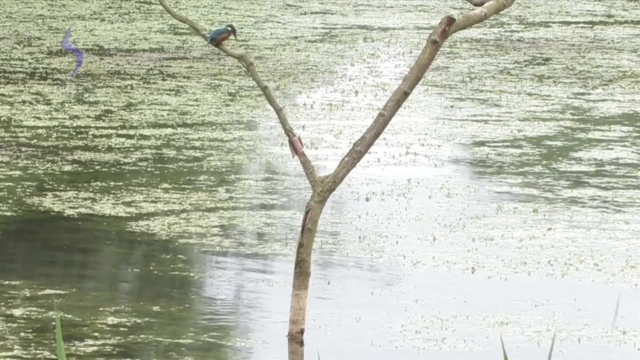 And though they themselves are harmless, they gain a degree of protection from their similarity to the dangerously armed wasps and bees. This does not, however, protect them from some particularly sharp-eyed insect-eating birds. Mimicry Feeding relationships can be either simple or complex. 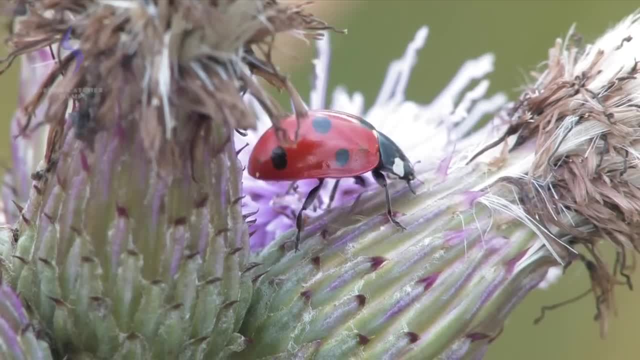 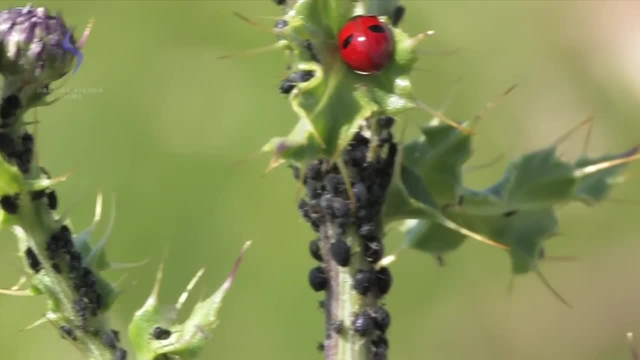 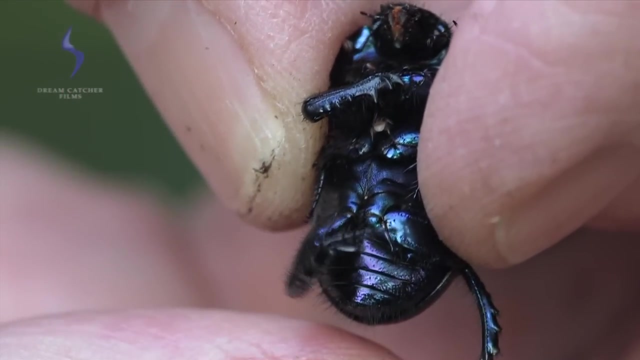 In a higher fauna. most predator populations are governed by the availability of prey. Prey levels are rarely limited solely by the impacts of the predator. On the other hand, parasitic predation can cause very dramatic declines in the availability of the host species. 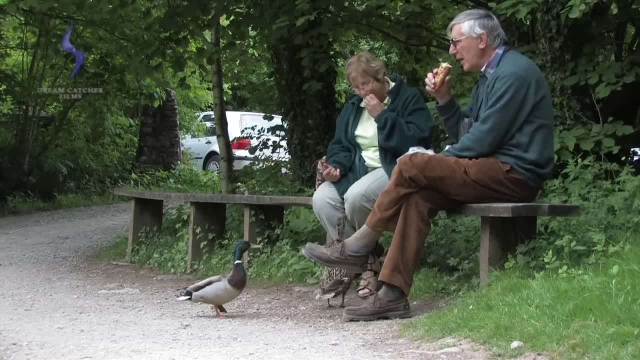 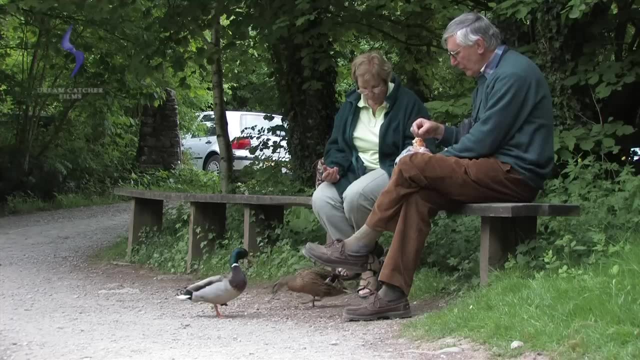 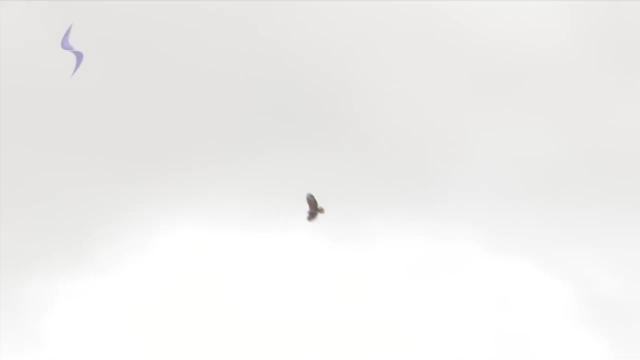 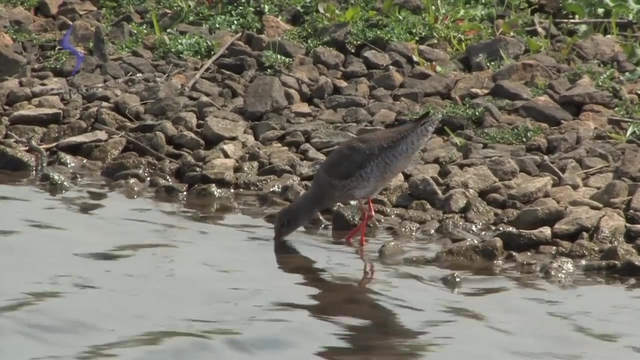 Except where man introduces an unpredictable variable, most ecosystems maintain a balance of populations, and change is normally a slow process. In those circumstances where species undergo dramatic population fluctuations, they normally do so on a predictable cycle. What is certainly true is that the health our natural environment determines its carrying capacity and biodiversity. 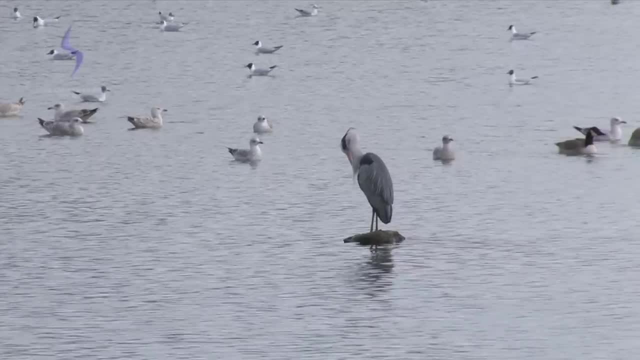 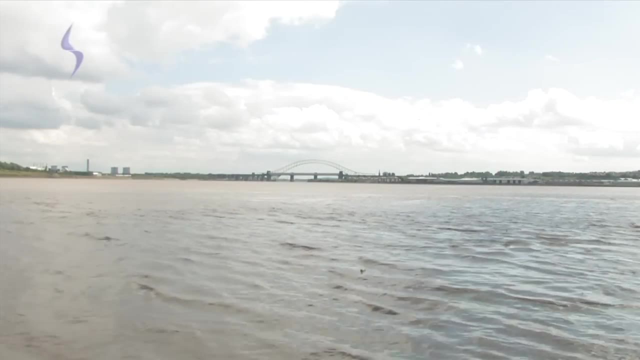 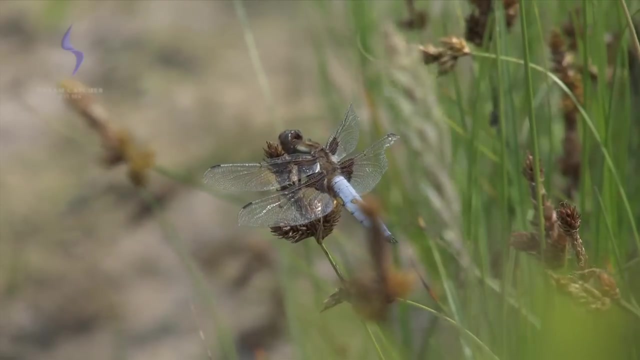 This in turn limits the variety and complexity of feeding relationships that can develop. The more biologically diverse an ecosystem is, then the greater will be the number and variety of predators present within it. Predators are an essential asset, playing a critical role in maintaining the health and balance of an ecosystem.